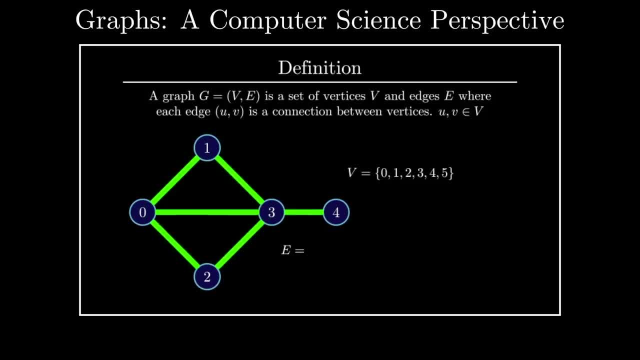 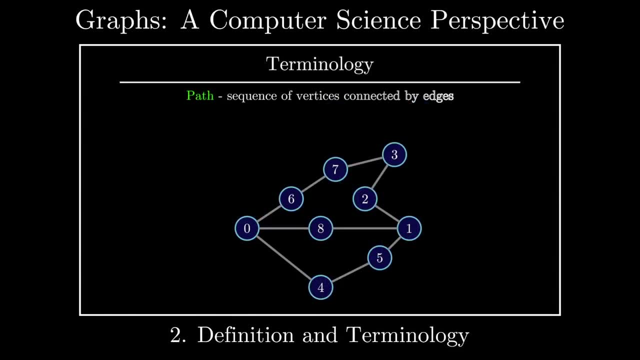 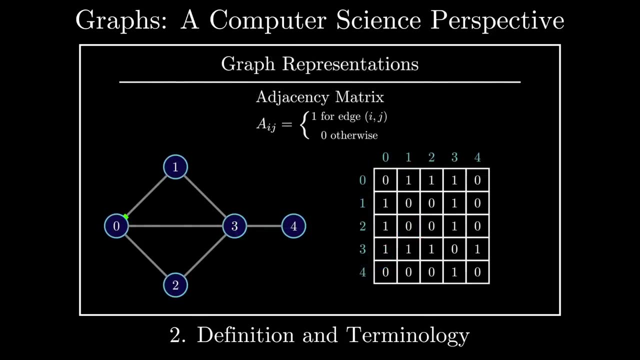 graph theory that we will then use to study fundamental graph algorithms. We'll first start with an important discussion on why we should even care about studying graphs, after which we'll formally define a graph and introduce important terminology used to communicate ideas about graphs. Then we'll talk about how computers might represent graphs as a data structure, And then I'll 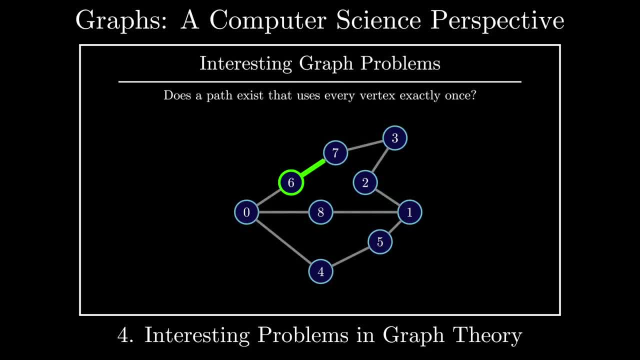 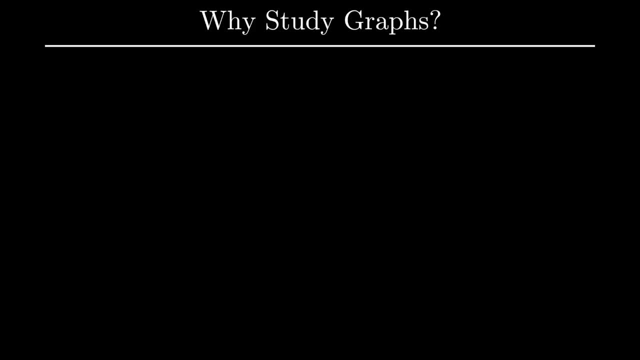 finish the video off with some interesting problems and questions around graphs that you can think about going forward. Let's first start with the most important question: Why should we care about graph theory? And the short answer to this is: graphs show up everywhere, sometimes in expected ways and also sometimes in surprising ways. 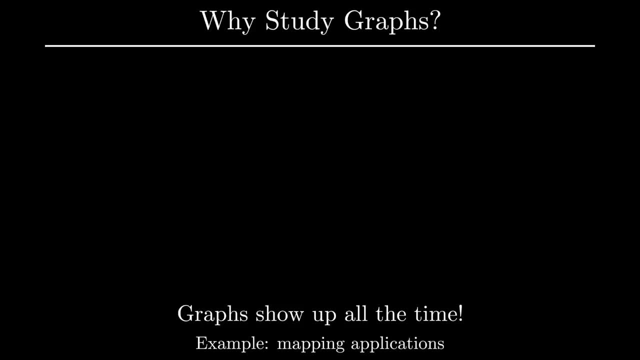 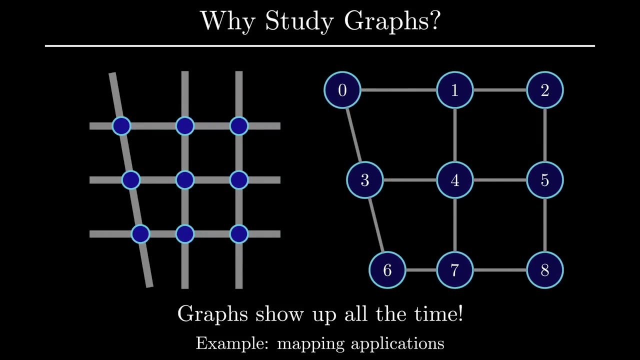 One of the most direct applications are in mapping and navigation applications. In any of these applications you often deal with roads and intersections, which can be naturally modeled as a graph, where each vertex represents an intersection and the edge between vertices signify the roads between intersections You could imagine navigation applications might be. 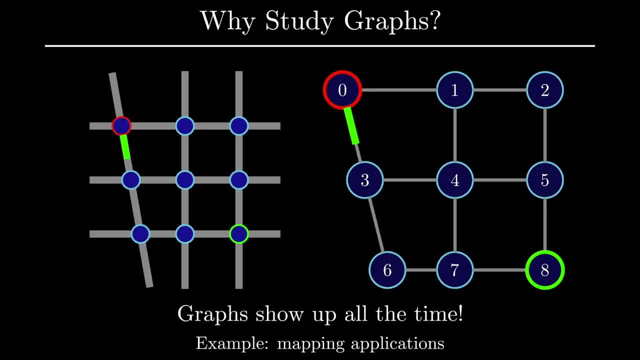 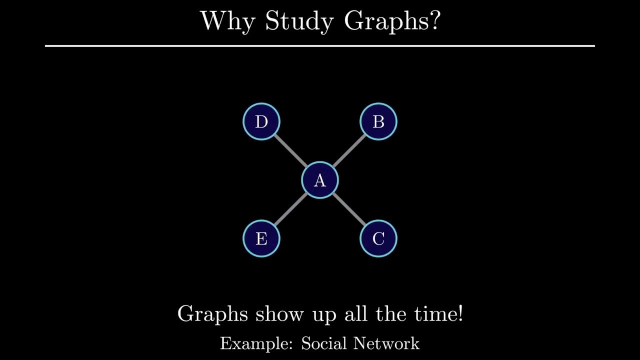 interested in the best route between a starting point and an ending point, and this problem naturally translates into many well-known graph theory problems. Another natural application of graphs is in social networks. In the context of this application, imagine: edges of a graph now represent friendships between people in a network where each node now 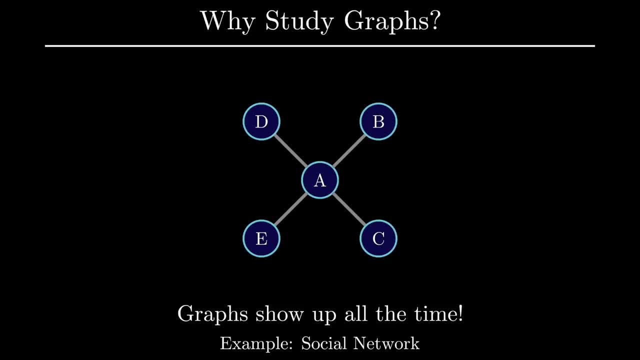 represents an individual. Suppose you are interested in a graph and you want to know what the graph looks like, then you might want to look at the graph of a person who has 4 friends. A natural way to solve this problem is to look at all of person A's friends. 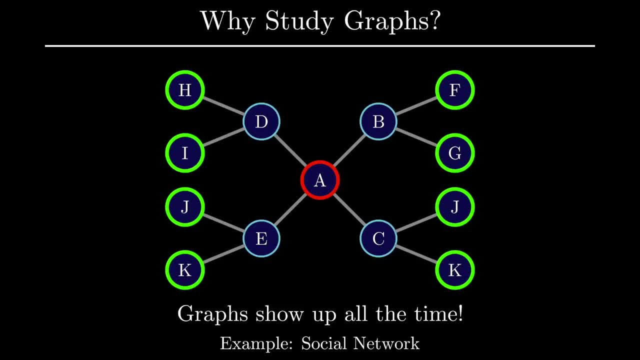 find friends of these friends and recommend them. These type of problems are easily modeled and solved with graph theory, So these are examples of applications where it's honestly not too surprising that something like graph theory shows up. but the neat thing about graph theory is that it also finds ways to show up. 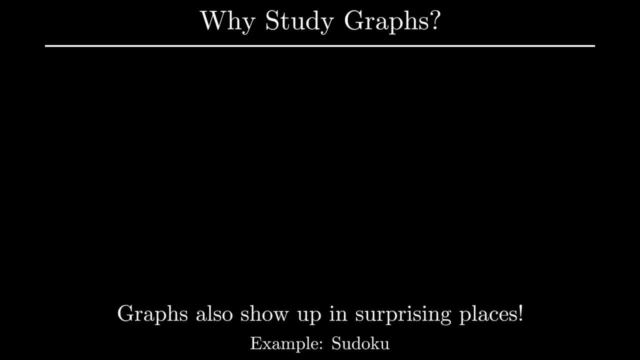 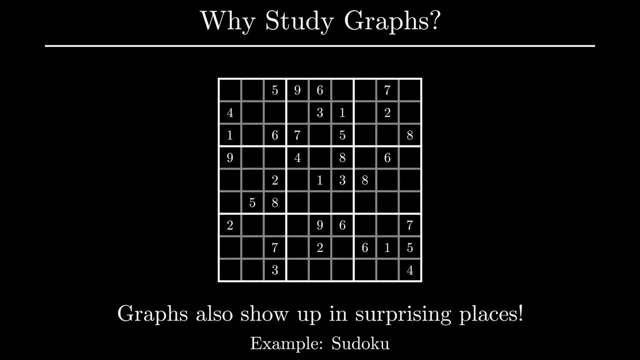 in the most unexpected places. Let's talk about Sudoku. That's right. I bet you didn't see that one coming. A lot of you have probably encountered a Sudoku puzzle at some point, but for those of you who haven't, here's a quick summary of how this puzzle works, so we're all on the same page. 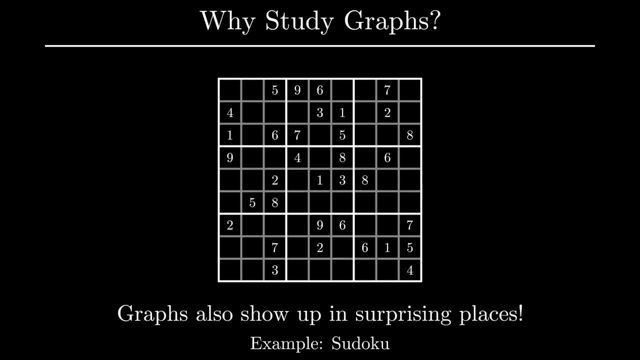 The goal of Sudoku is to fill missing entries of a 9 by 9 grid with numbers 1 through 9, but with a few constraints. The first constraint is that each 3 by 3 subgrid cannot have repeated numbers. The next constraint is that each row must have: 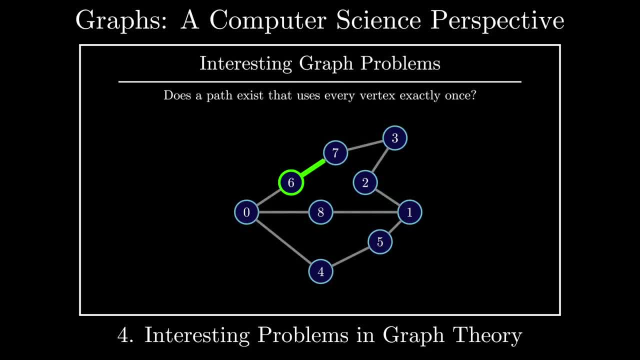 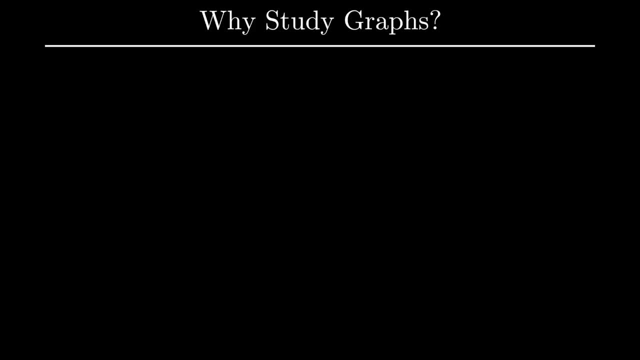 finish the video off with some interesting problems and questions around graphs that you can think about going forward. Let's first start with the most important question: Why should we care about graph theory? And the short answer to this is: graphs show up everywhere, sometimes in expected ways and also sometimes in surprising ways. 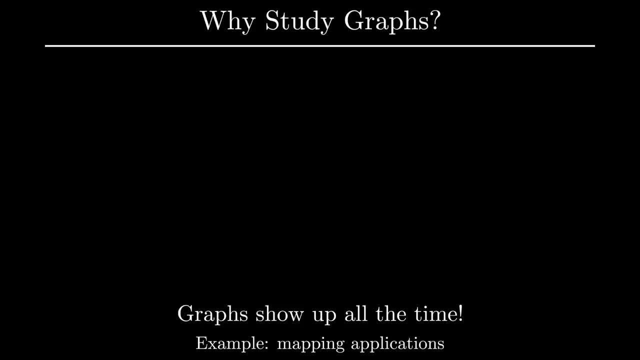 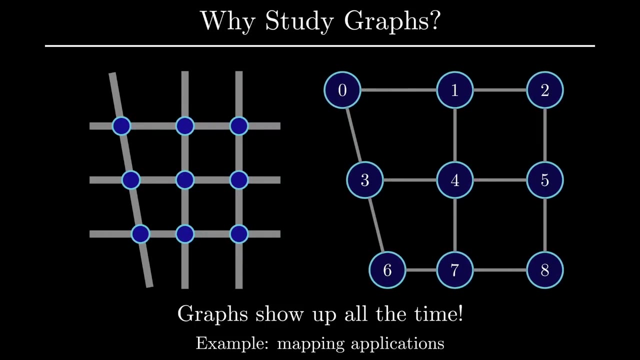 One of the most direct applications are in mapping and navigation applications. In any of these applications you often deal with roads and intersections, which can be naturally modeled as a graph, where each vertex represents an intersection and the edge between vertices signify the roads between intersections You could imagine navigation applications might be. 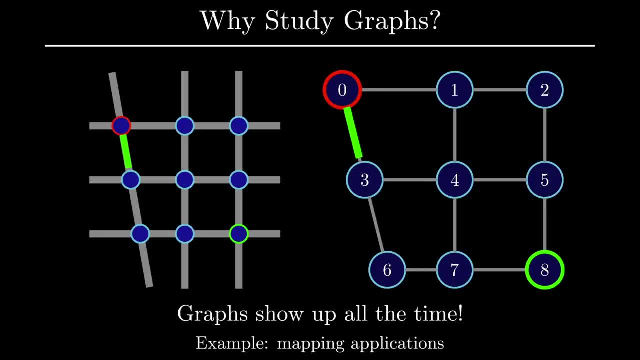 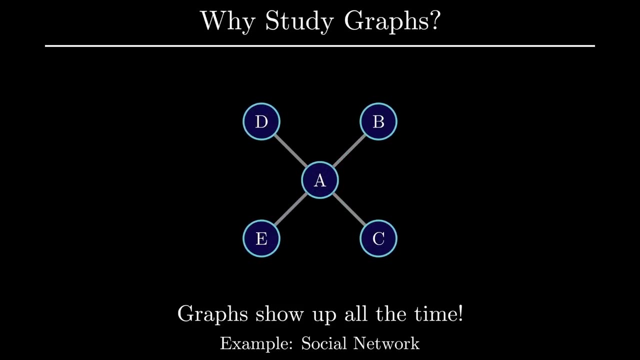 interested in the best route between a starting point and an ending point, and this problem naturally translates into many well-known graph theory problems. Another natural application of graphs is in social networks. In the context of this application, imagine: edges of a graph now represent friendships between people in a network where each node now 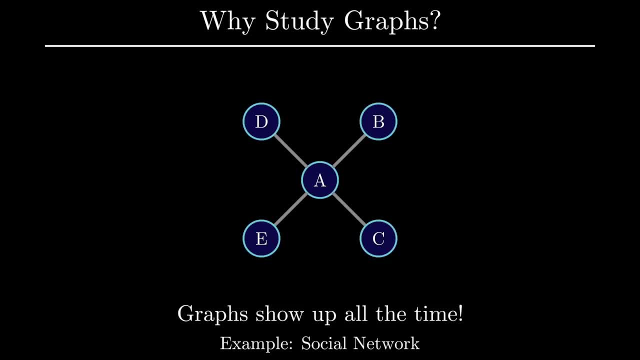 represents an individual. Suppose you are interested in a graph and you want to know what the graph looks like, then you might want to look at the graph of a person who has 4 friends. A natural way to solve this problem is to look at all of person A's friends. 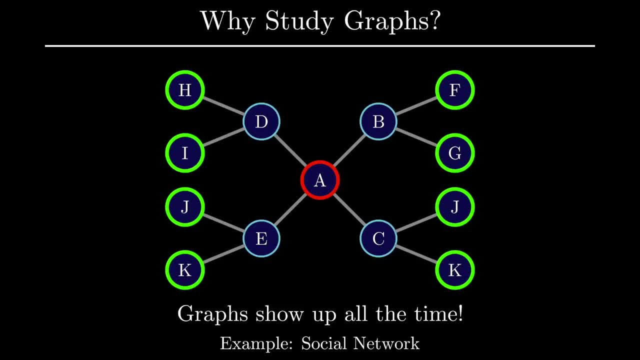 find friends of these friends and recommend them. These type of problems are easily modeled and solved with graph theory, So these are examples of applications where it's honestly not too surprising that something like graph theory shows up. but the neat thing about graph theory is that it also finds ways to show up. 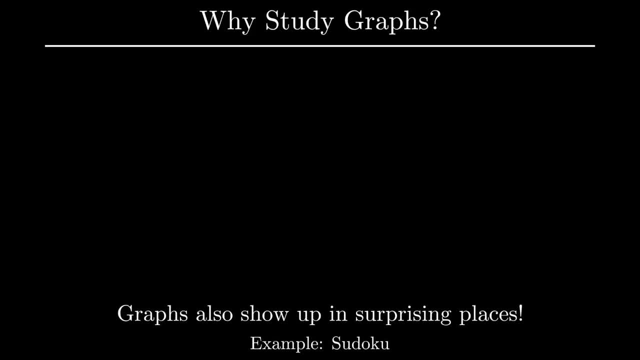 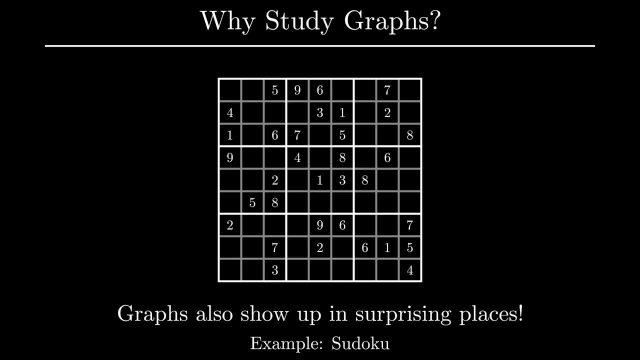 in the most unexpected places. Let's talk about Sudoku. I bet you didn't see that one coming. A lot of you have probably encountered a Sudoku puzzle at some point, but for those of you who haven't, here's a quick summary of how this puzzle works. 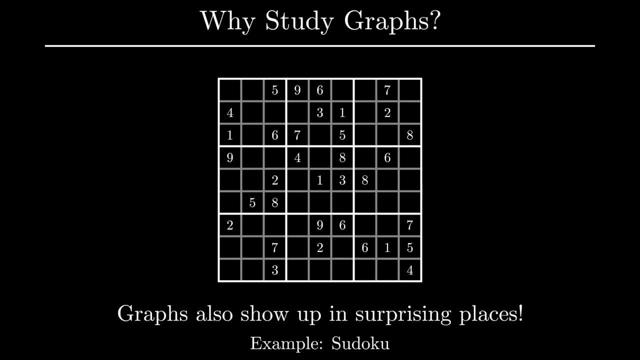 so we're all on the same page. The goal of Sudoku is to fill missing entries of a 9x9 grid with numbers 1 through 9, but with a few constraints. The first constraint is that each 3x3 subgrid 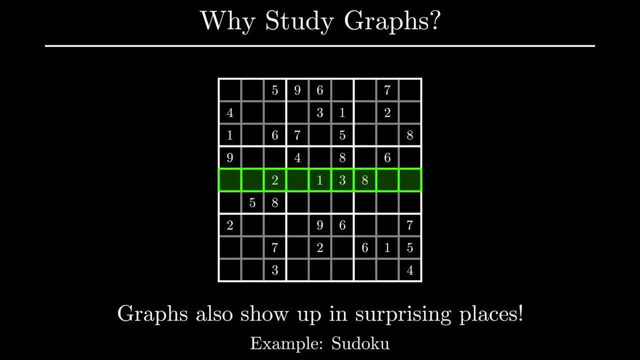 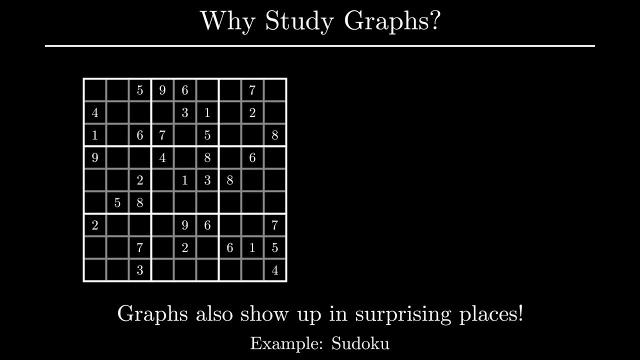 cannot have repeated numbers. The next constraint is that each row must have unique entries, and the last constraint puts a similar limitation on the columns, in which all entries of a column must be unique. So it turns out that computers can solve Sudoku puzzles efficiently using graph theory. The graph here is quite subtle, but it does exist. 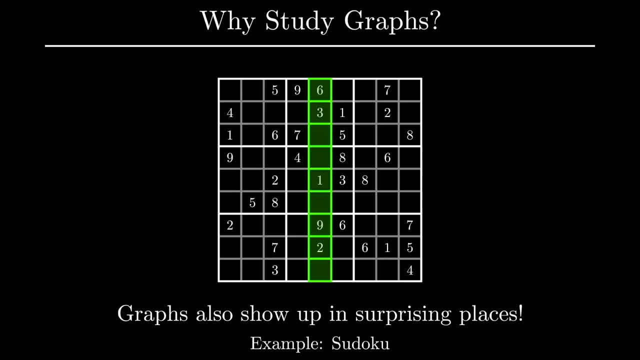 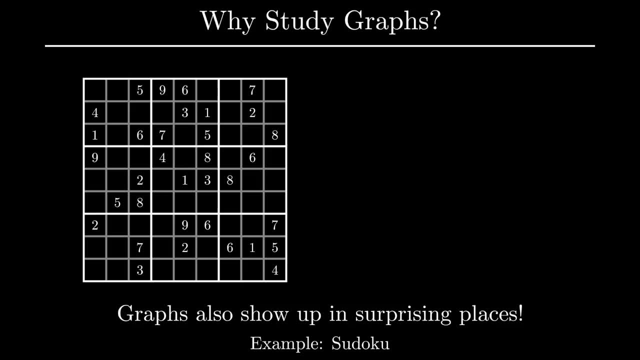 unique entries, and the last constraint puts a similar limitation on the columns, in which all entries of a column must be unique. So it turns out that computers can solve Sudoku puzzles efficiently using graph theory. The graph here is quite subtle, but it does exist. 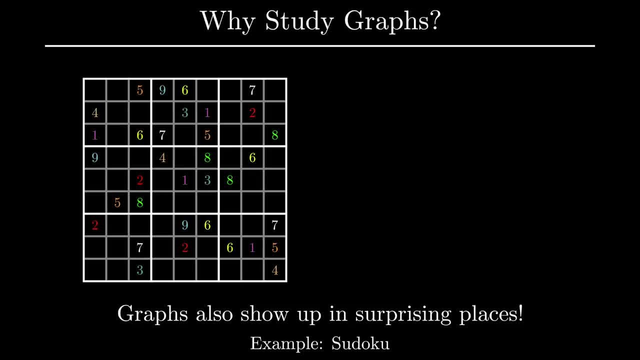 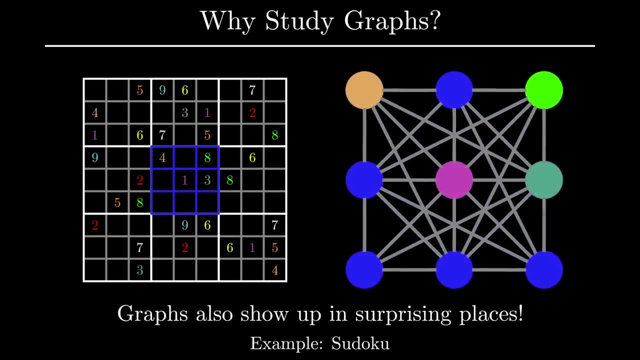 What we're going to do is we're going to assign each number a color and then construct a graph as follows: For each 3 by 3 grid, we'll fill out the unknown entries with the respective color for that number and assign one color to all unknown entries. The constraint here: 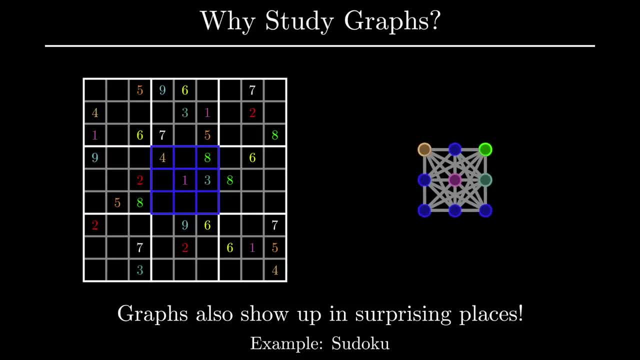 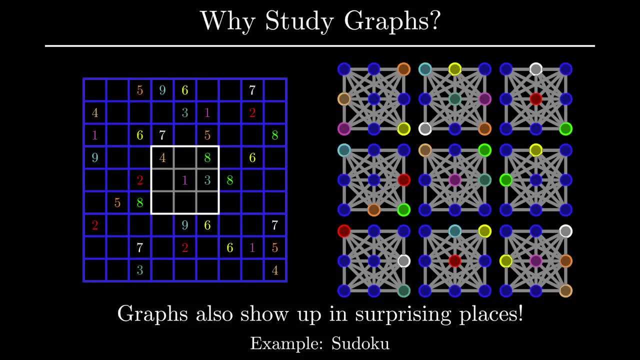 is that all of these 9 nodes as a group must have unique colors. We can then extend this mapping to all other 3 by 3 grids and create the following graph: Now we still have to take care of the other constraints. We can connect the graph along. 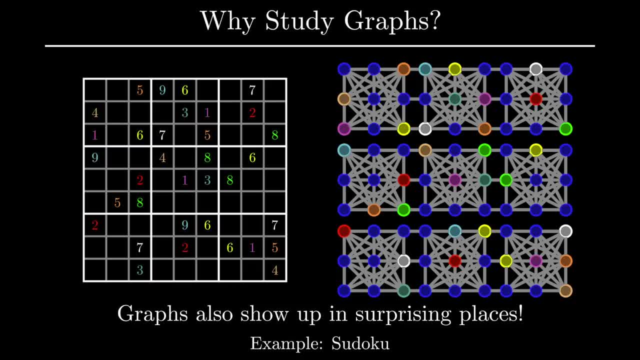 each row to represent the idea that every row in the graph must have a unique color and we can do the same connections along columns for that respective constraint. Now we have a graph theory problem where we attempt to find colors assigned to vertices that satisfies all the laid out constraints And it turns out that this is actually a 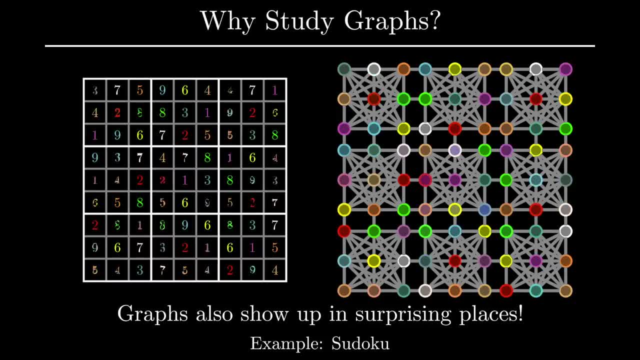 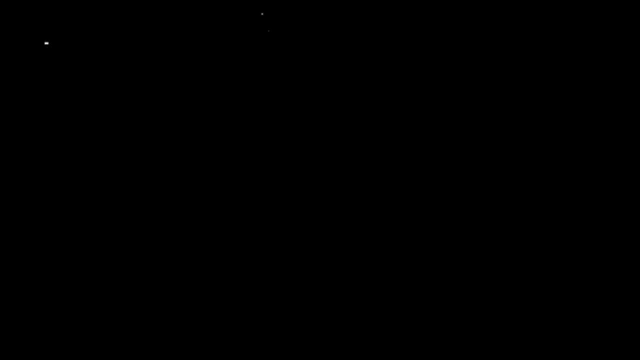 well known graph problem. that graph theory provides an elegant algorithm for and once we find a set of colors, we have a solution to the Sudoku puzzle. Let's now proceed to formally define a graph. A graph is a set of vertices and edges, where each 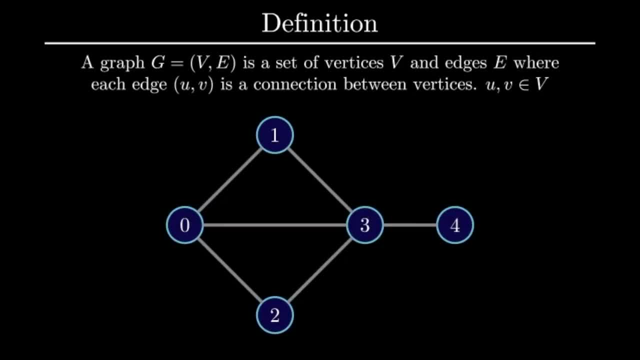 edge is a connection between vertices. The way we usually denote an edge in a graph is by referring to it as a pair of vertices And, as mentioned before, vertices and nodes are just different names for the same constraint. Now we can define a graph where each edge has the same connection. 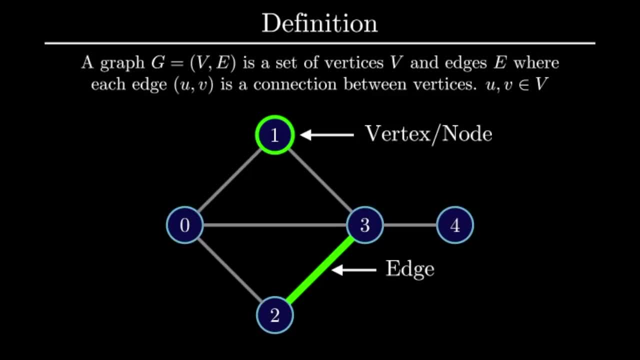 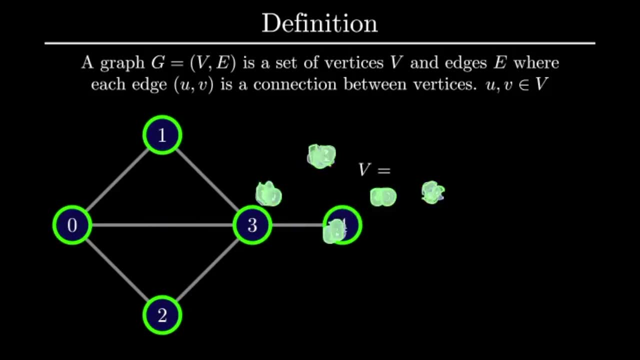 that we will use interchangeably when discussing graphs. If you're forced to mathematically write down a definition of a graph, we can use set notation For this particular graph. the vertex set looks like this, and our set of edges would be denoted with this notation. 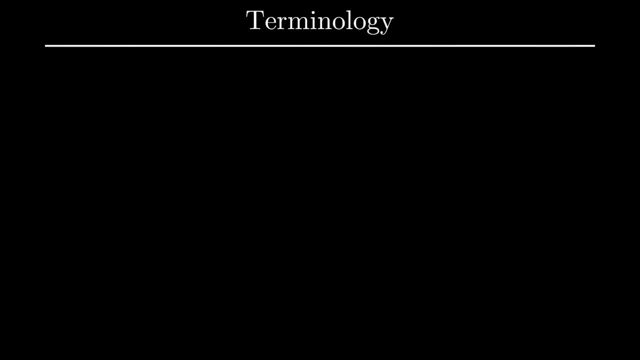 Let's now define some important terminology that you'll see over and over again when talking about graphs. The first important term is the concept of neighbors in a graph. Formally, two vertices are neighbors if an edge connects them. Here's an example. 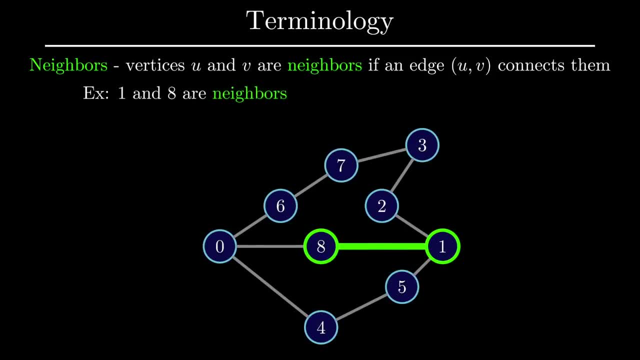 Vertices one and eight of this graph are neighbors, since they are connected by an edge. One thing that we will often query a graph for is all neighbors of a particular vertex. For example, if we were to ask for all the neighbors of node zero, the result would be the following set: 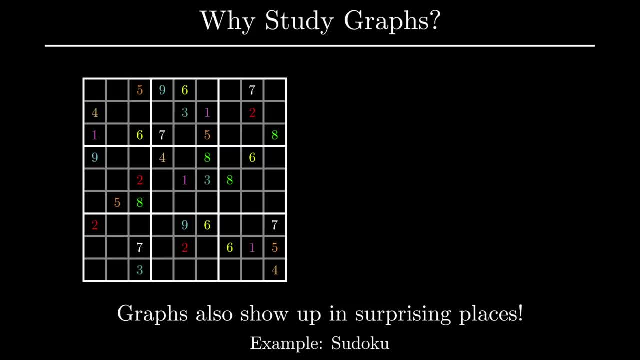 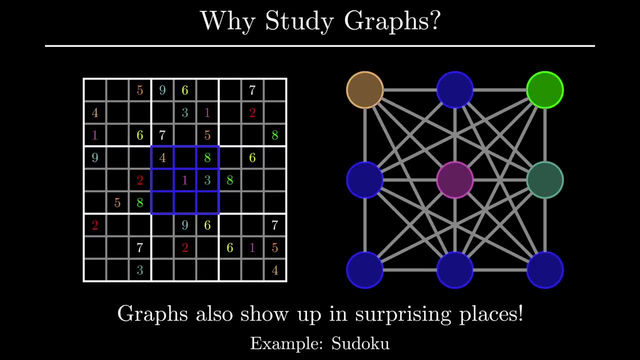 What we're going to do is we're going to assign each number a color and then construct a graph as follows: For each 3x3 grid, we'll fill out the unknown entries with the respective color for that number and assign one color to all unknown entries. The constraint here is that 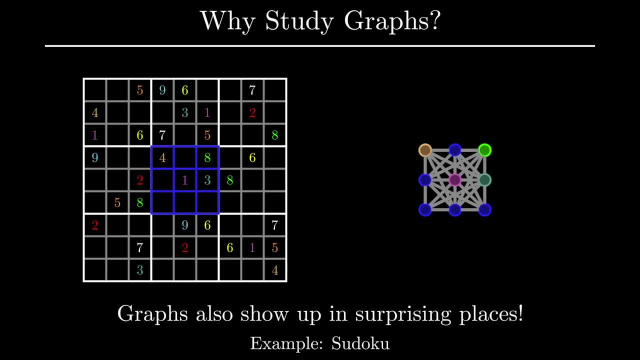 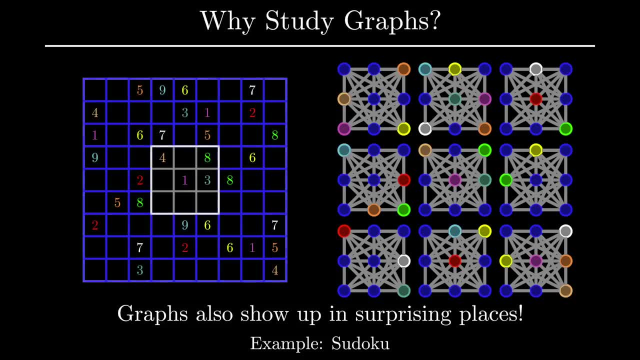 all of these 9 nodes as a group must have unique colors. We can then extend this mapping to all the 3x3 grids and create the following graph: Now we still have to take care of the other constraints. We can connect the graph along each row to represent the idea that every row in the 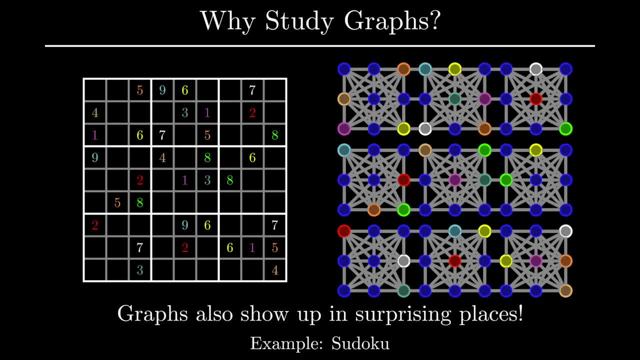 graph must have a unique color and we can do the same connections along columns for that respective constraint. Now we have a graph theory problem where we attempt to find colors assigned to vertices that satisfies all the laid out constraints and turns out that this is actually 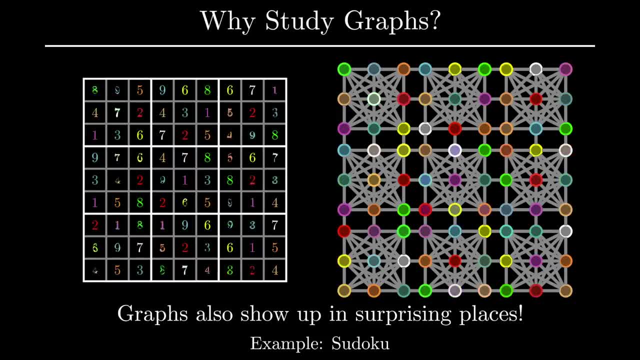 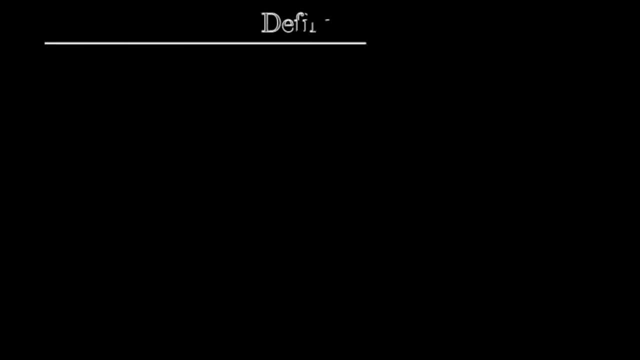 a graph problem. that graph theory provides an elegant algorithm for and once we find a set of colors, we have a solution to the Sudoku puzzle. Let's now proceed to formally define a graph. A graph is a set of vertices and edges, where each 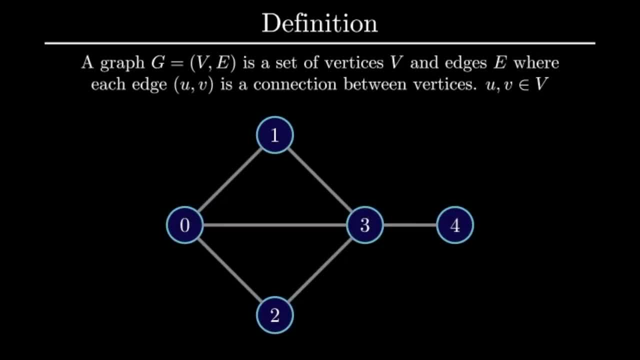 edge is a connection between vertices. The way we usually denote an edge in a graph is by referring to it as a pair of vertices And, as mentioned before, vertices and nodes are just different names for the same concepts that we're going to use to define a graph. So let's start with a graph. 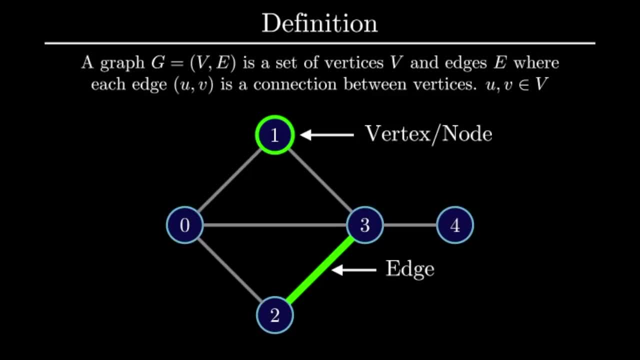 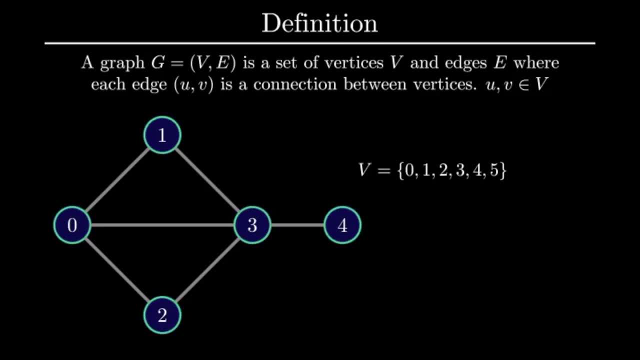 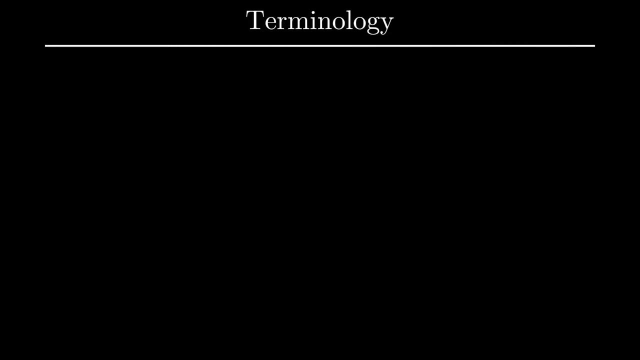 For this particular graph, the vertex set looks like this and our set of edges would be denoted with this notation. Let's now define some important terminology that you will see over and over again when talking about graphs. The first important term is the concept of 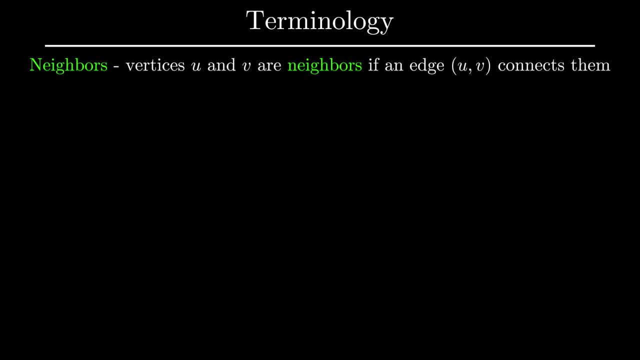 neighbors in a graph. Formally, two vertices are neighbors if an edge connects them. Here's an example: Vertices 1 and 8 of this graph are neighbors, since they are connected by an edge. One thing that we will often query a graph for is all neighbors of a particular vertex. 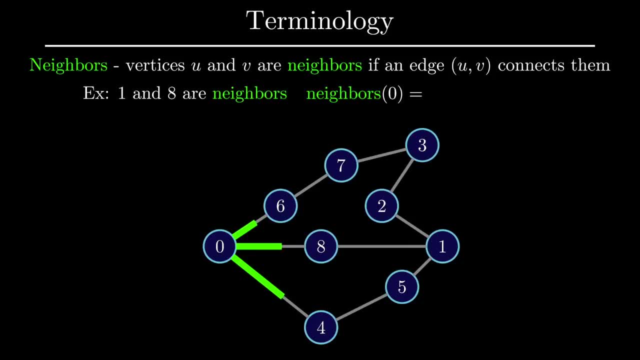 For example, if we were to ask for all the neighbors of node 0,, the result would be the following: set of three nodes: Nodes 4, 6, and 8.. A related concept is the degree of a vertex. A degree of a specific vertex is equal to the. 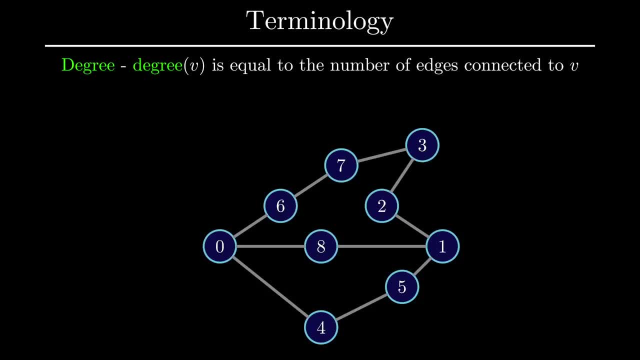 number of edges connected to that vertex or, equivalently, the number of neighbors. As per this definition, the degree of vertex 0 would be 3, and the degree of vertex 3 would be 2.. Let's now talk about paths. 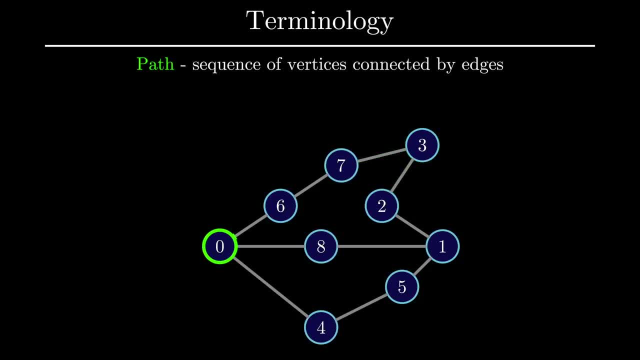 Paths are simply defined as a sequence of vertices connected by edges. Most of the paths that we deal with will be paths with unique vertices. For example, one path from vertex 0 to vertex 2 is shown here, and all vertices in the path only show up once, which is what we will assume most of the time. 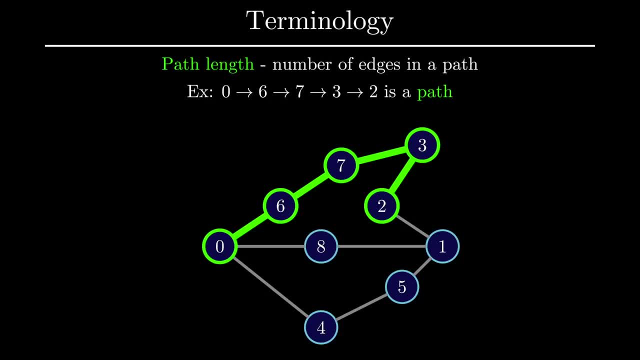 One feature of paths is that they have respective lengths. A path length is simply defined as the number of edges in a path. In this example, the path length we have here would be 4.. A related idea to a path is the concept of a cycle. A cycle is defined as a path that starts. 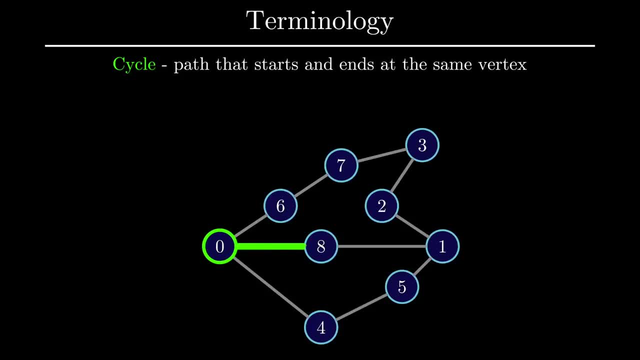 and ends at the same vertex. One key note about cycles is that all cycles are paths, but not all paths are necessarily cycles. There are several cycles in this graph. Here's an example of a cycle that begins at vertex 0 and ends at vertex 0.. 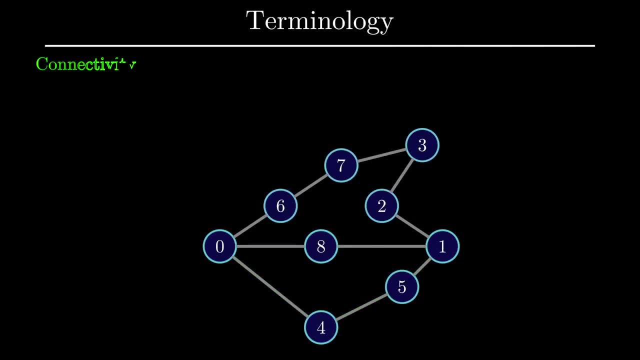 The last term I want to talk about is the concept of connectivity, which can be used in this example. The first context is with respect to two specific vertices. Two vertices are connected if a path exists between them. The second context you may encounter connectivity is when it is applied to a general graph. 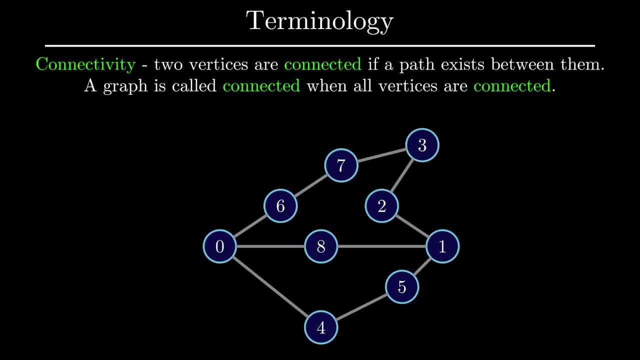 A graph is connected when all vertices are pairwise connected. In other words, a path exists between all pairs of vertices. This graph is an example of a connected graph, since if you pick any two vertices in the graph, we can identify a path between them. However, 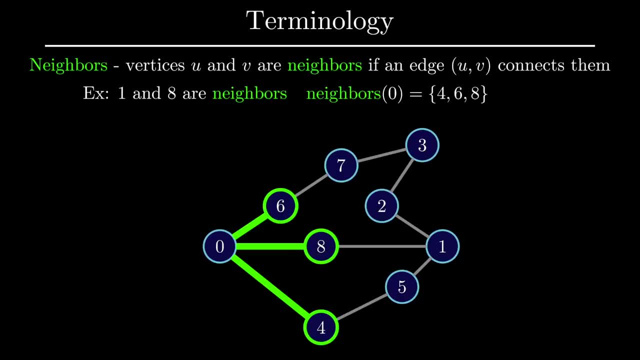 of three nodes: nodes four, six and eight. A related concept is the degree of a vertex. A degree of a specific vertex is equal to the number of edges connected to that vertex or, equivalently, the number of neighbors. As per this definition, the degree of vertex zero. 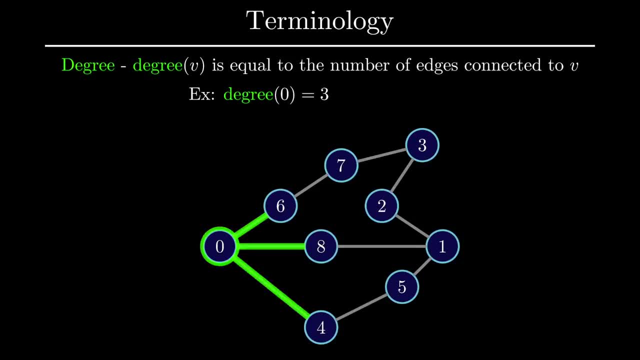 would be three, and the degree of vertex three would be two. Let's now investigate a graph. Let's now talk about paths. Paths are simply defined as a sequence of vertices connected by edges. Most of the paths that we deal with will be paths with. 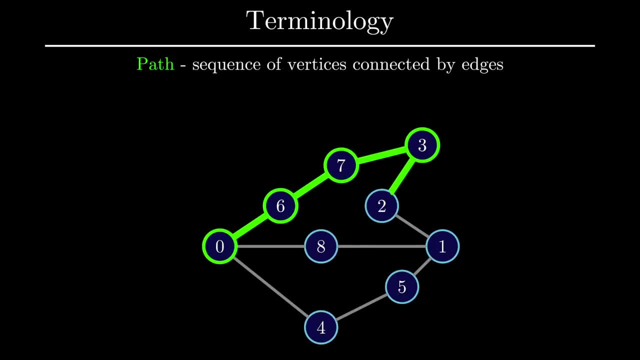 unique vertices. For example, one path from vertex 0 to vertex 2 is shown here, and all vertices in the path only show up once, which is what we will assume most of the time. One feature of paths is that they have respective lengths. A path 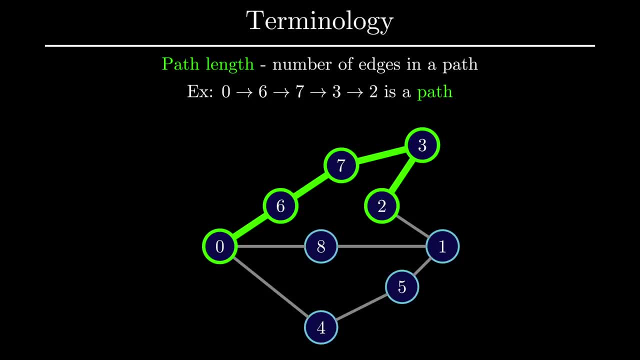 length is simply defined as the number of edges in a path. In this example, the path among we have here would be 4.. A related idea to a path is the concept of a cycle. A cycle is defined as a path that starts and ends at the same vertex. 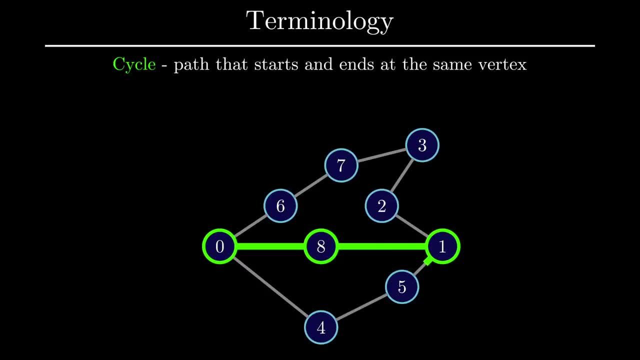 One key note about cycles is that all cycles are paths, but not all paths are necessarily cycles. There are several cycles in this graph. Here's an example of a cycle that begins at vertex 0 and ends at vertex 0. The last term I want to talk about is the concept of connectivity, which can be used in several contexts. 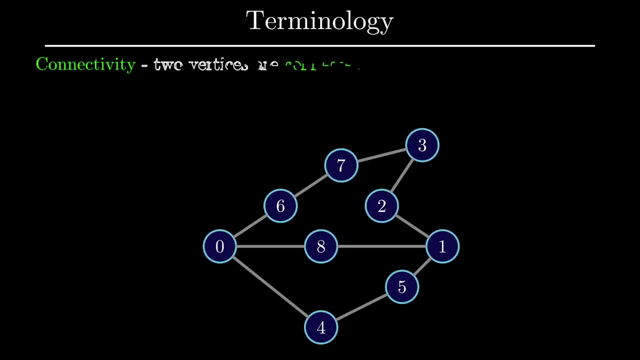 The first context is with respect to two specific vertices. Two vertices are connected if a path exists between them. The second context you may encounter connectivity is when it is applied to a general graph. A graph is connected when all vertices are pairwise connected. In other words, a path exists between all pairs of vertices. This graph is an example of a connected. 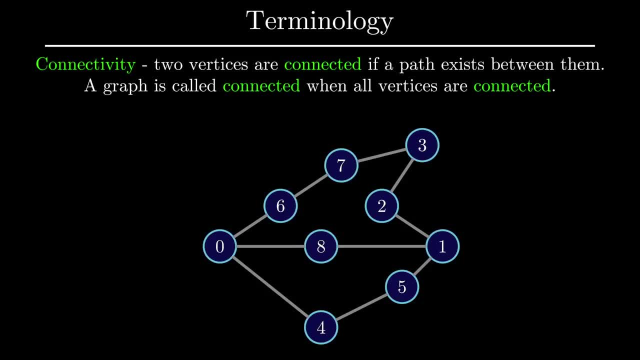 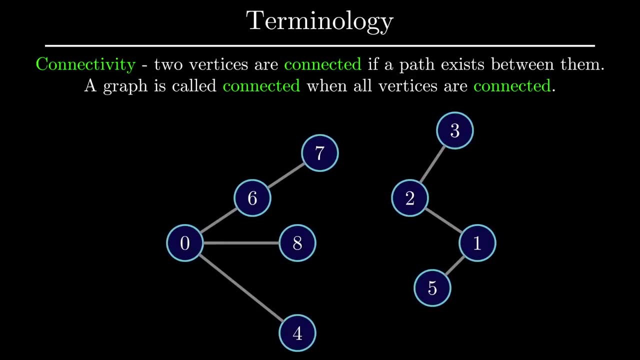 graph, since if you pick any two vertices in the graph, we can identify a path between them. However, if we change up the graph a little bit, we now have an example of a graph that is not connected. Now it's easy to see that no path exists between several pairs of vertices. This naturally leads to: 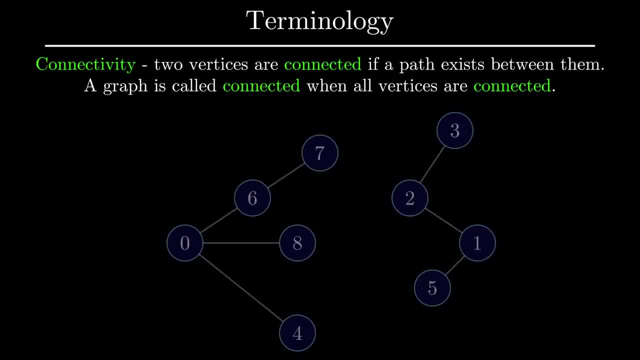 if we change up the graph a little bit, we now have an example of a graph that is not connected. Now it's easy to see that no path exists between several pairs of vertices. This naturally leads to a third context that connectivity can be applied. 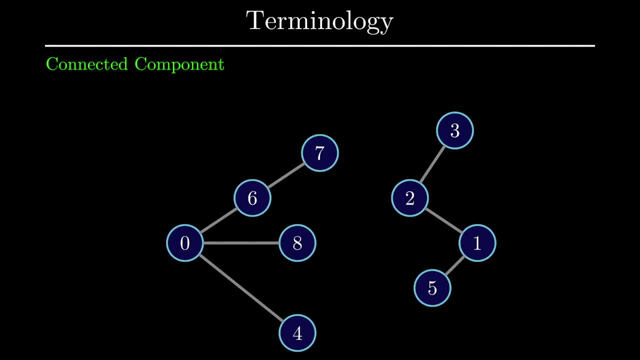 which is the idea of a connected component. A connected component is a subset of vertices of the graph that is connected. For example, in this graph, we have two connected components, the first being the following set of vertices and then the remaining vertices of the graph. 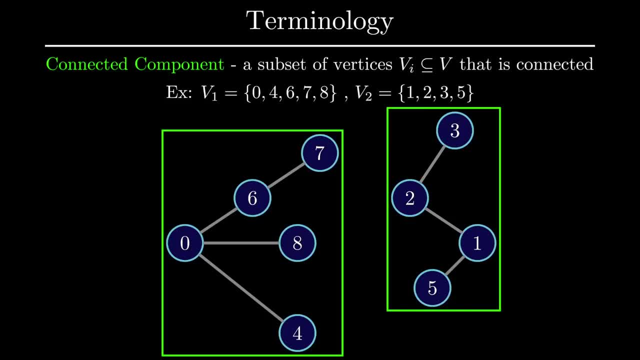 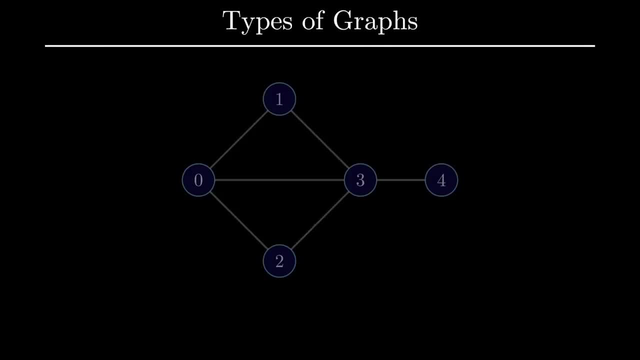 Let's now transition to the types of graphs that you may encounter. The main graph we've seen so far is specifically called an undirected graph, where, for example, if I have an edge connecting vertex 0 to vertex 1, it's kind of implied that I also have an edge from vertex 1 to vertex 0.. 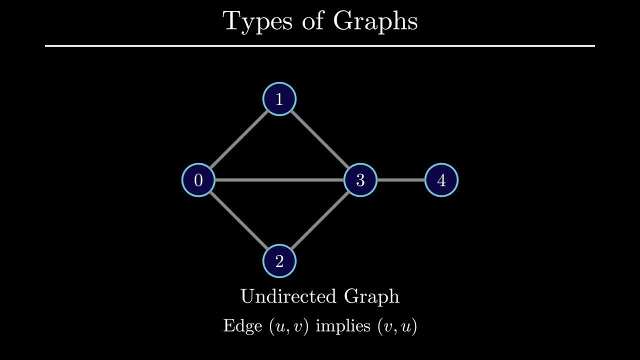 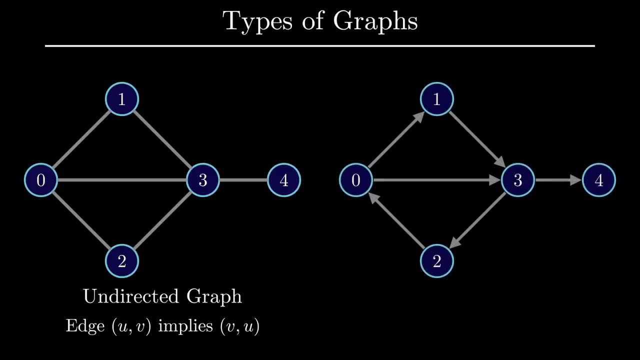 A graph where this would not be the case is called a directed graph, where now edges are usually connected to vertices 1 and vertex 2.. The second connected component is a graph that is connected to the second connected component. This graph is called a unidirectional graph or unidirectional. 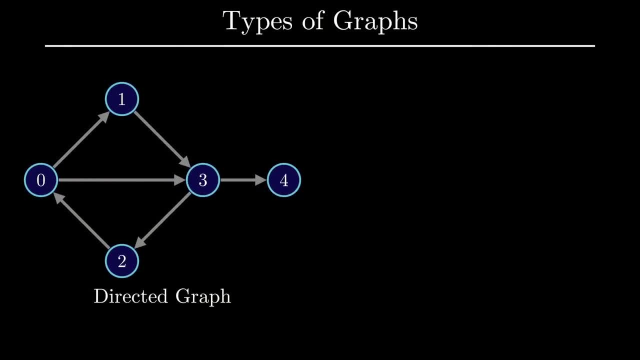 Directed graphs also have their own classes. This particular graph has a cycle, so we can be more specific by referring to this graph as a directed cyclic graph. On the other hand, if a graph is directed and contains no cycles, we refer to that specifically as a directed acyclic graph. 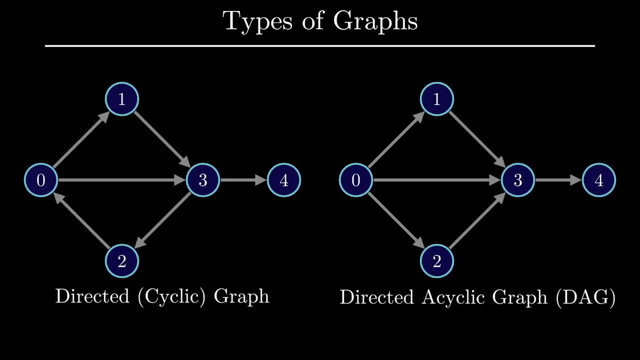 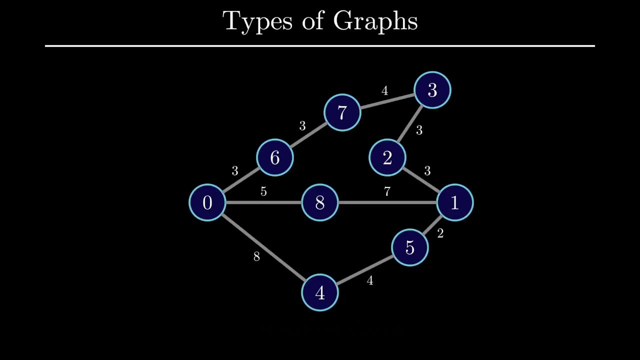 which is a specific subset of graphs that has been studied quite rigorously, since they show up in all sorts of interesting problems. The third connected component is a weighted graph. This graph is unique because each edge is now not treated equally and some edges might have a larger weight than others. 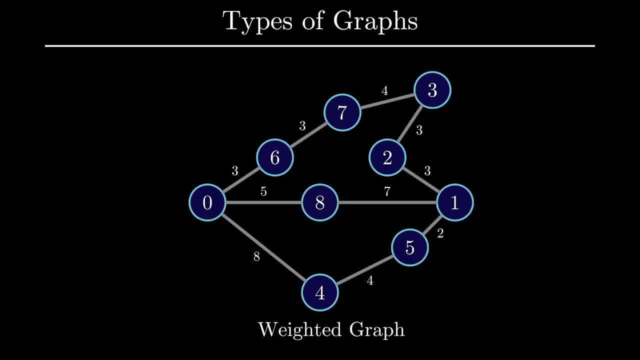 This can naturally model interesting metrics like traffic distances on maps and many other ideas. Another important class of graphs is trees. Trees have three key properties: All trees are connected and acyclic. Removing an edge from a tree will disconnect the entire graph. 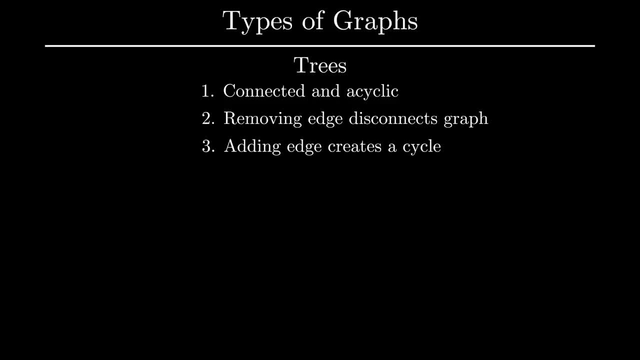 and, furthermore, adding any single edge to a tree will create a cycle. These are three valid examples of trees and I encourage you to take a second, pause the video and confirm that all of these properties hold. Personally, I find verifying the second and third properties surprisingly satisfying. 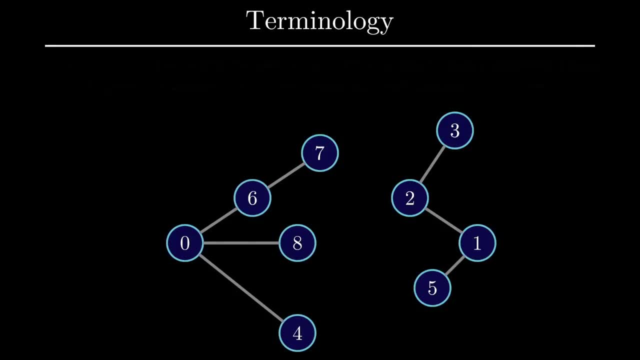 a third context that connectivity can be applied, which is the idea of a connected component. A connected component is a subset of vertices of the graph that is connected. For example, in this graph we have two connected vertices, connected components, the first being the following set of vertices and then the remaining. 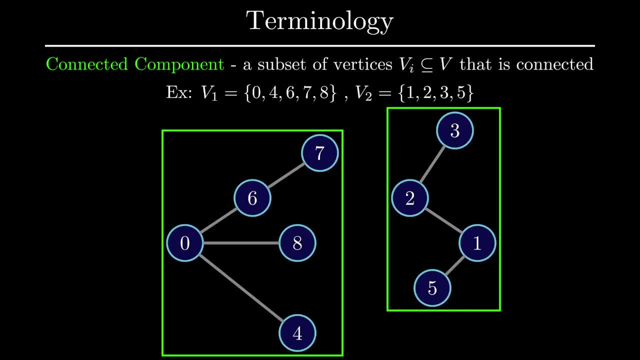 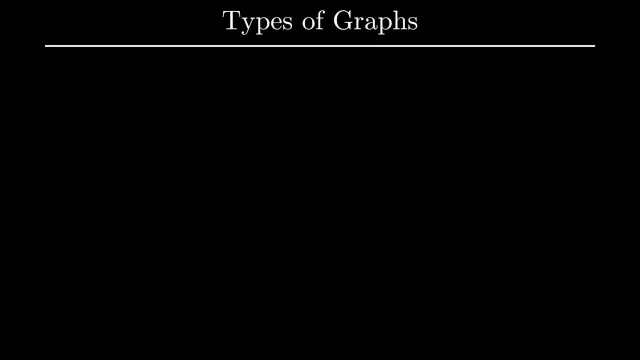 vertices of the graph form the second connected component. Let's now transition to the types of graphs that you may encounter. The main graph we've seen so far is specifically called an undirected graph where, for example, if I have an edge connecting vertex 0 to vertex 1, it's kind of implied that I also have an 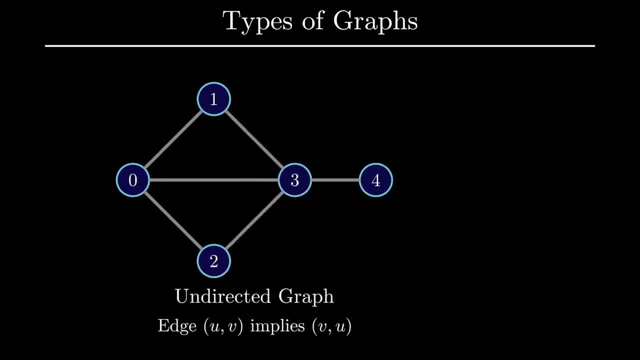 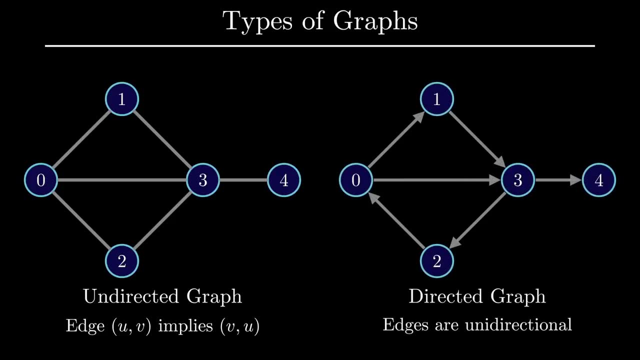 edge from vertex 1 to vertex 0.. A graph where this would not be the case is called a directed graph, where now edges are unidirectional. Directed graphs also have their own classes. This particular graph has a cycle, so we can be more specific by referring to this graph. 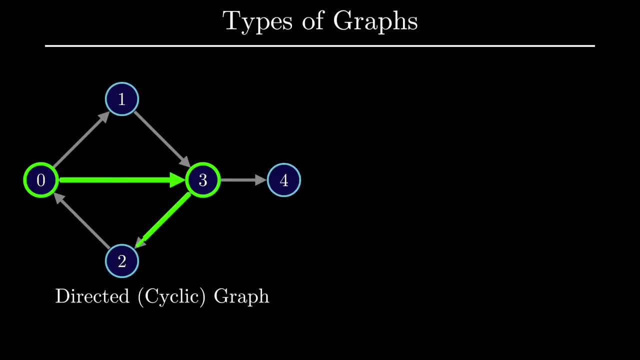 as a directed cyclic graph. On the other hand, if a graph is directed and contains no cycles, we refer to that specifically as a directed acyclic graph, Which is a specific subset of graphs That has been studied quite rigorously, since they show up in all sorts of interesting problems. 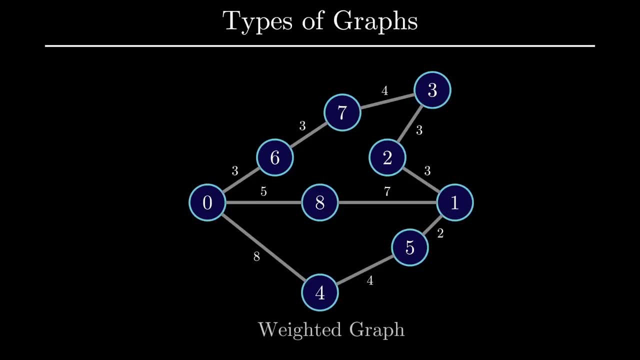 Another important graph is a weighted graph. This graph is unique because each edge is now not treated equally and some edges might have a larger weight than others. This can naturally model interesting metrics like traffic distances on maps and many other ideas. Another important class of graphs is trees. 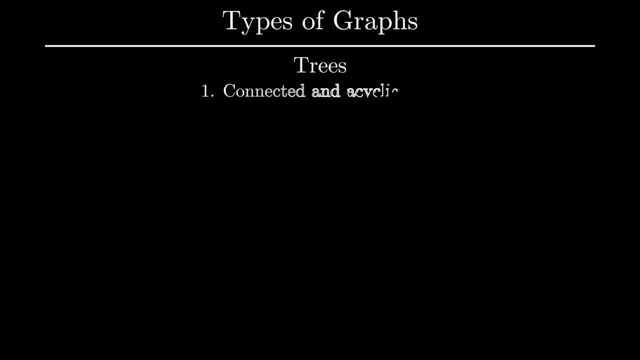 Trees have three key properties. All trees are connected and acyclic. Removing an edge from a tree will disconnect the entire graph and, furthermore, adding any single edge to a tree will create a cycle. These are three valid examples of trees and I encourage you to take a second pause: the 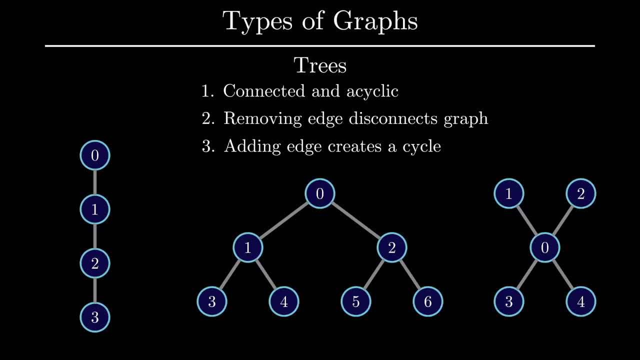 video and confirm that all of these properties hold. Personally, I find verifying the second and third properties surprisingly satisfying. Really emphasizes how fragile a tree's structure is, which I think is kind of cool. Let's now move on to some more hands-on ideas. 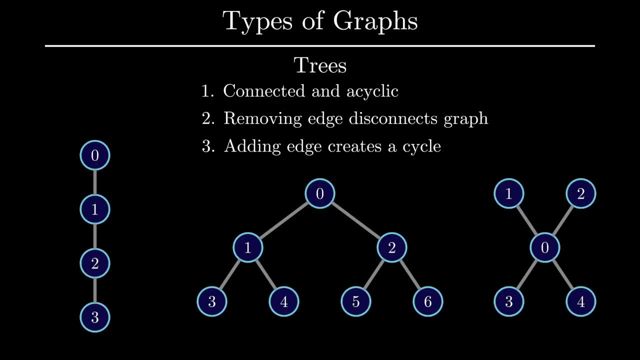 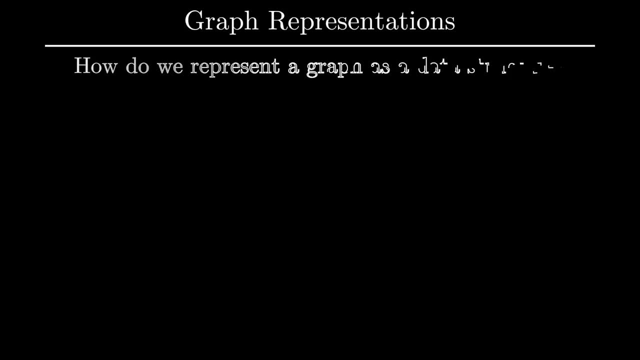 It really emphasizes how fragile a tree's structure is, which I think is kind of cool. Let's now move on to some more hands-on ideas. How does a computer represent a graph as a data structure? Take, for example, the following graphs: 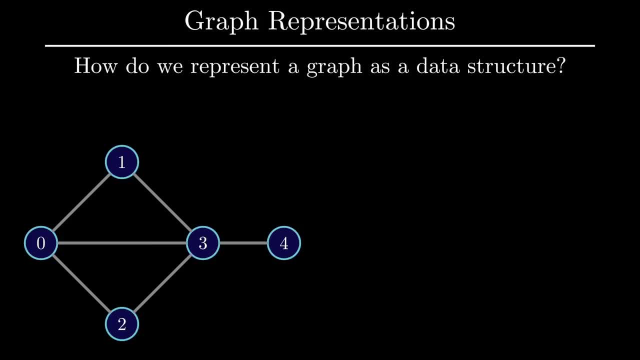 How would you go about organizing the information in this graph on a computer? It turns out that there are several accepted ways to do this, and some of them are better than others, depending on the context. The first idea, that is quite natural, is to map vertices to one another through a matrix. 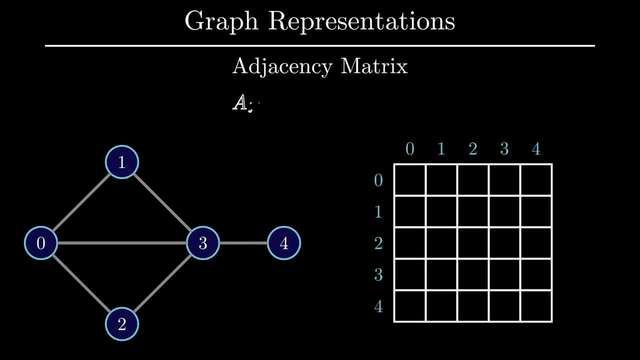 which we formally call an adjacency matrix. The rules for creating this matrix are fairly intuitive. If an edge between node i and j exists, we will indicate this with an entry 1 in our matrix. Otherwise, the entry will be 0.. Following these rules, this is what our adjacency matrix looks like for this graph. 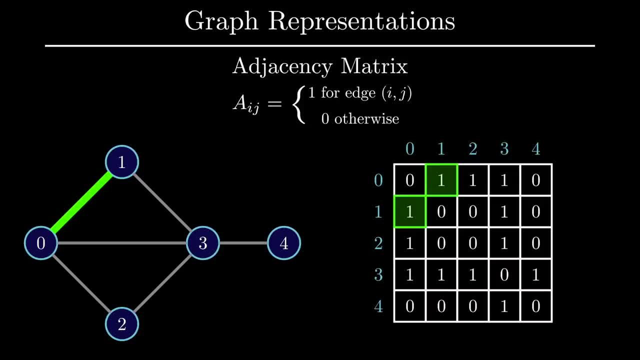 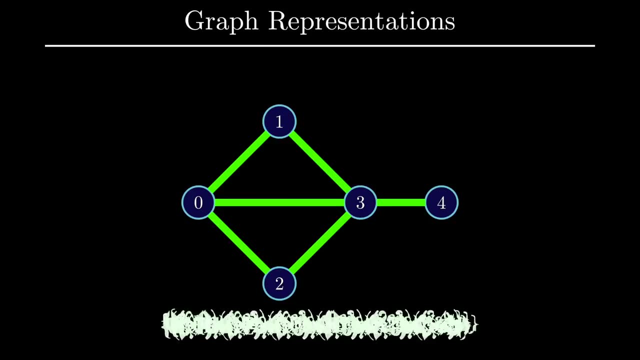 Notice that each edge creates two entries. since this is an undirected graph, Make sure you take a moment to understand the mapping we have here. The second valid representation of a graph is actually fairly simple. We take all the edges and construct a set with each edge as follows. 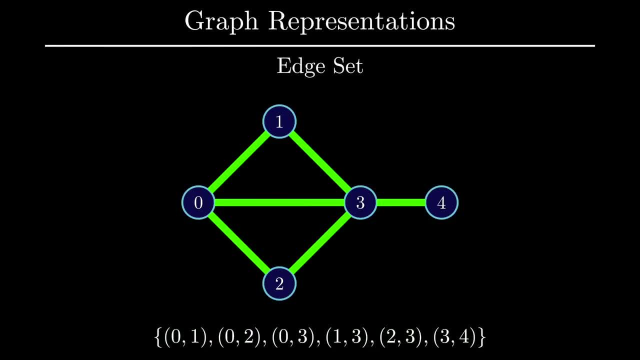 This representation is called an edge set and it also contains all the information about vertices and edges that you would need for a graph. However, this representation is not as common because it's a little hard to extract information about vertices of a graph using this particular representation. 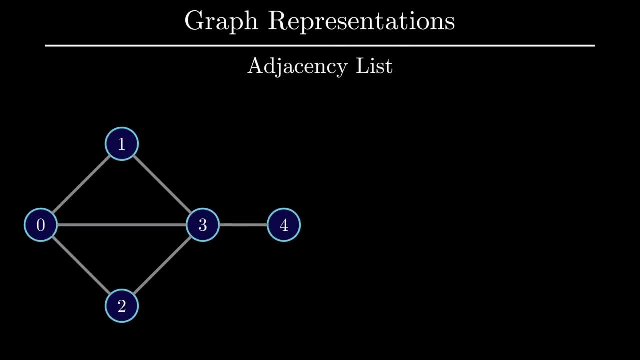 The third representation of a graph is called an adjacency list, and this is actually the most common representation used. The idea works as follows: We take each vertex and map the vertex to a list of its neighbors. For example, node 0 has three neighbors, specifically nodes 1,, 2, and 3,. 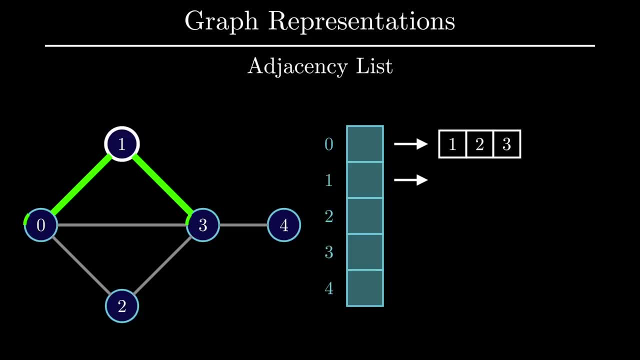 so we map it to a list containing those values. The rest of the list is constructed in a similar way. The nice thing about this representation is that it gives us an easy access to neighbors of a particular node, which is a tool that will be immensely useful in graph algorithms. 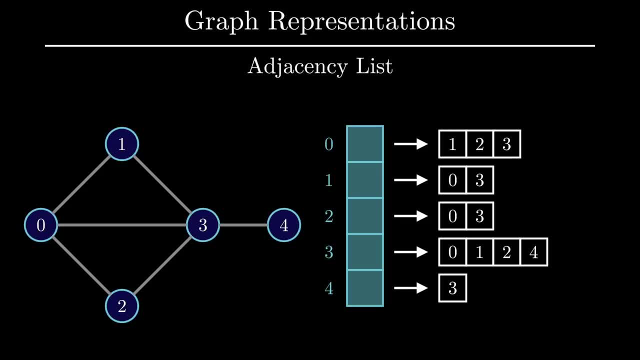 Furthermore, this representation exploits the fact that most graphs in the real world are going to be sparse, meaning that we have a large number of vertices, with each vertex having relatively few edges. For example, in a social network, it would actually make the most sense to have 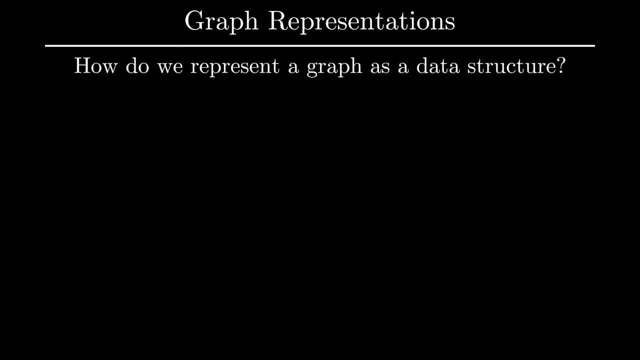 How does a computer represent a graph? How does a computer represent a graph? How does a computer represent a graph as a data structure? Take, for example, the following graphs: How would you go about organizing the information in this graph on a computer? Turns out that there are several accepted ways to do this, and some of them are better. 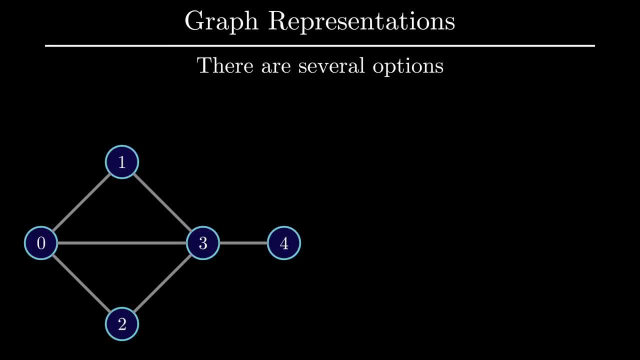 than others, depending on the context. The first idea, that is quite natural, is to map vertices to one another through a matrix, which we formally call an adjacency matrix. The rules for creating this matrix are fairly intuitive. If an edge between node i and node j exists, we will indicate this with an adjacent matrix. 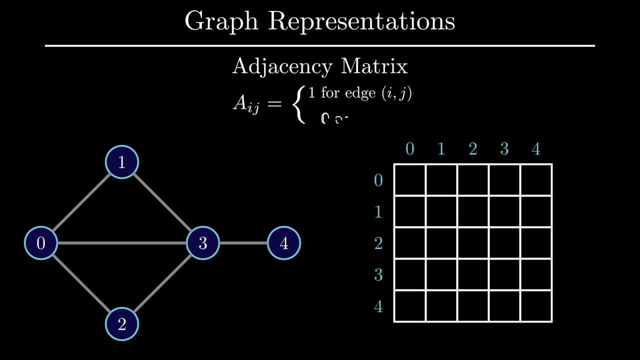 If an edge between node i and node j exists, we will indicate this with an adjacent matrix. The rules for creating this matrix are fairly intuitive. If an edge between node i and node j exists, we will indicate this with an adjacent matrix. We will enter: an자를 will be one in our matrix, otherwise the entry will be zero. 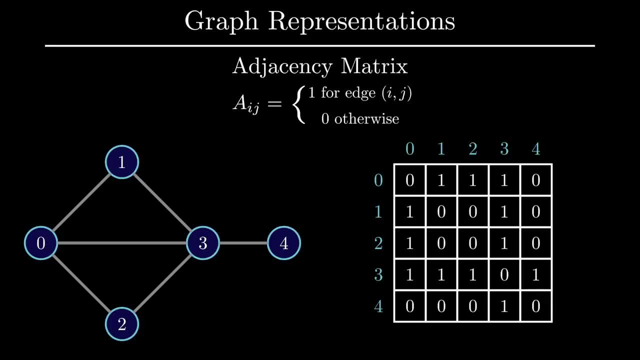 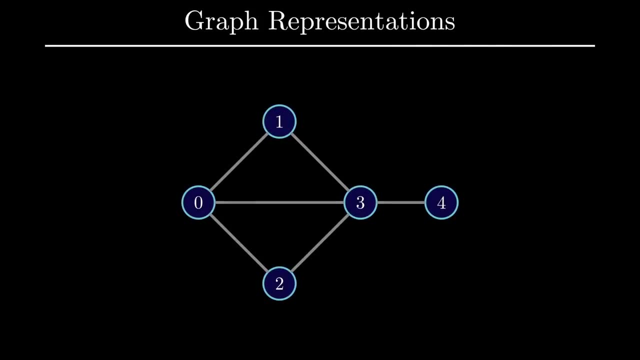 Following these rules. this is what our adjacency matrix looks like for the revised graph. Notice that each edge creates two entries. since this is an undirected graph, Make sure you take a moment to understand the mapping we have here. The second valid representation of a graph is actually fairly simple. 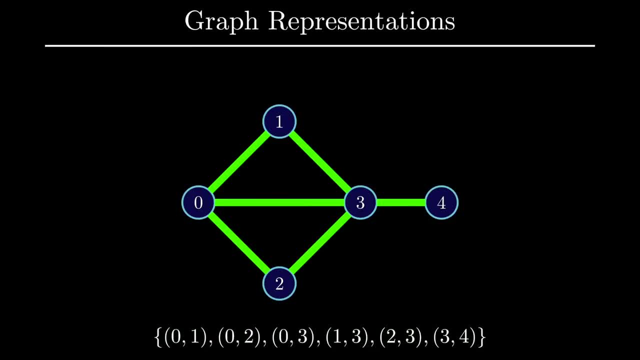 We take all the edges and construct a set with each edge as follows: edge set. and it also contains all the information about vertices and edges that you would need for a graph. However, this representation is not as common because it's a little hard to extract. 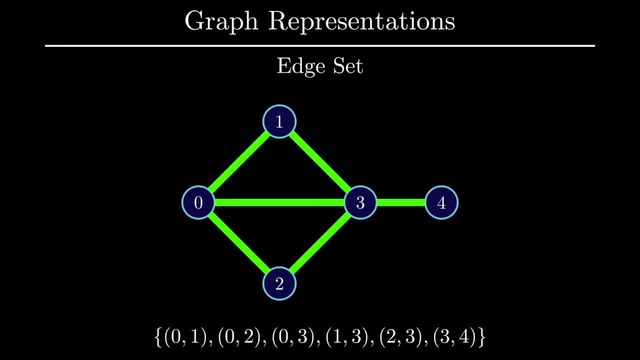 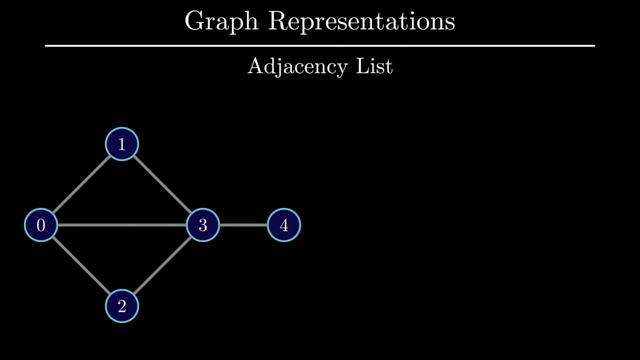 information about vertices of a graph using this particular representation. The third representation of a graph is called an adjacency list, and this is actually the most common representation used. The idea works as follows: We take each vertex and map the vertex to a list of its neighbors. 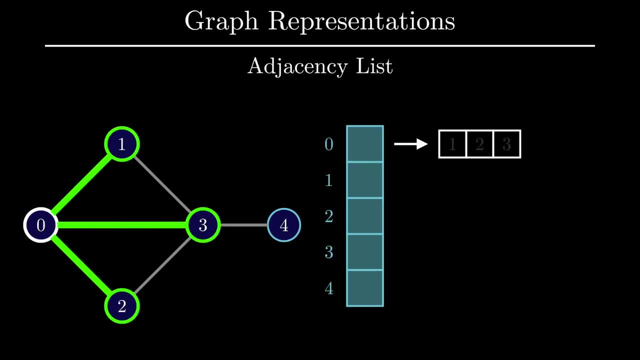 For example, node 0 has three neighbors, specifically nodes 1,, 2, and 3, so we map it to a list containing those values. The rest of the list is constructed in a similar manner. Nice thing about this representation is that it gives us an easy access. 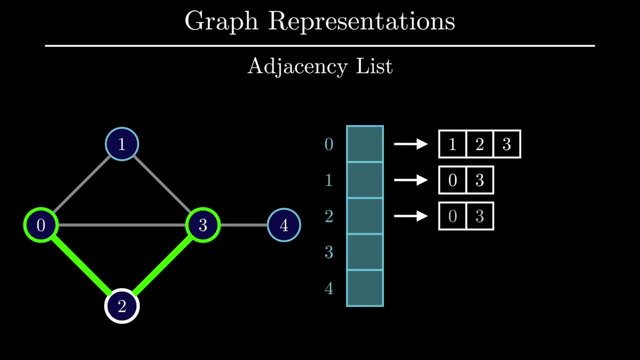 to neighbors of a particular node, which is a tool that will be immensely useful in graph algorithms. Furthermore, this representation exploits the fact that most graphs in the real world are going to be sparse, meaning that we have a large number of vertices with even better numbers of vertices that we can map to. 在形囲一些点. 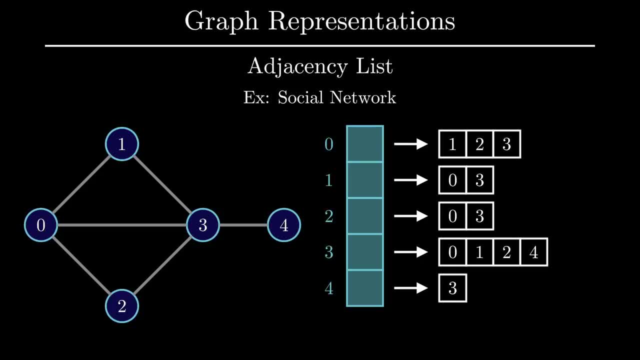 For example in a social network. it would actually make the most sense to have this representation, since there are gonna be billions of nodes, but each node is unlikely to have more than a few thousand edges. An adjacency matrix for a graph like that would take way too much memory. 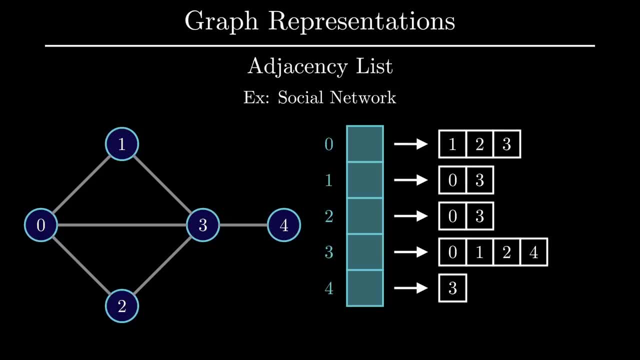 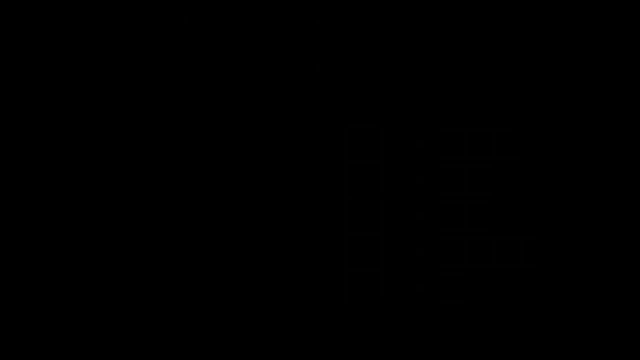 but with an adjacency list it's much more manageable. For this reason, in future videos we will primarily use adjacency lists as a way to represent graphs. The final thing I want to do in this video is to discuss some of the interesting problems. 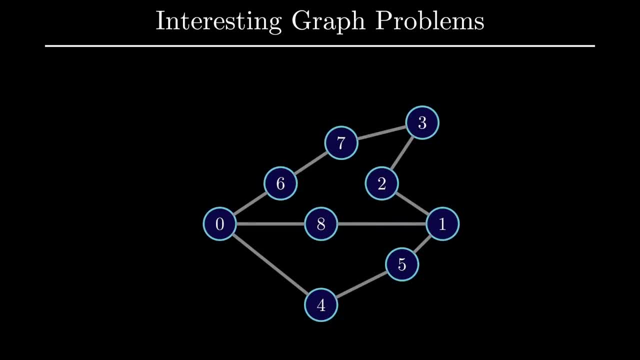 and questions you may find in graph theory. In future videos we'll show you how you can apply graph algorithms to solve many of these problems. A fairly standard problem that you'll likely encounter all the time revolves around connectivity between two vertices, For example. it's easy for us to see 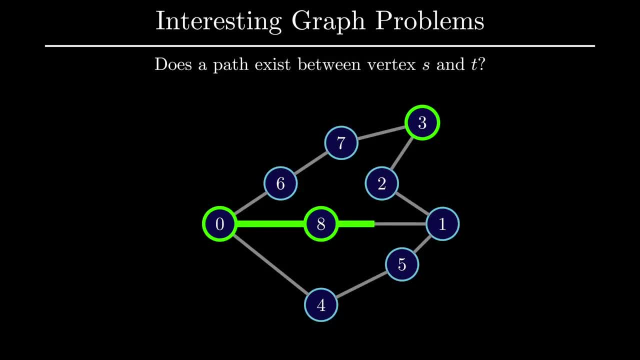 that vertices zero and three have many paths between them. but what sort of algorithms can we use to allow a computer to efficiently solve this problem? We can naturally extend this problem to ask if an entire graph is then connected. There are a variety of efficient algorithms. 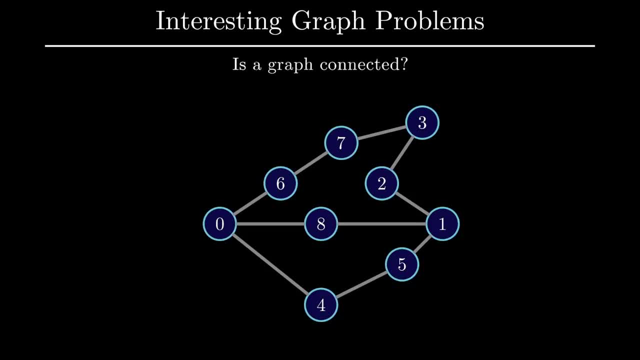 to solve these problems that we will cover in the next few videos. Another interesting problem in graph theory is the shortest path problem. Specifically, what is the path of the least length between two vertices For this particular graph? here's the shortest path between vertices zero and three. 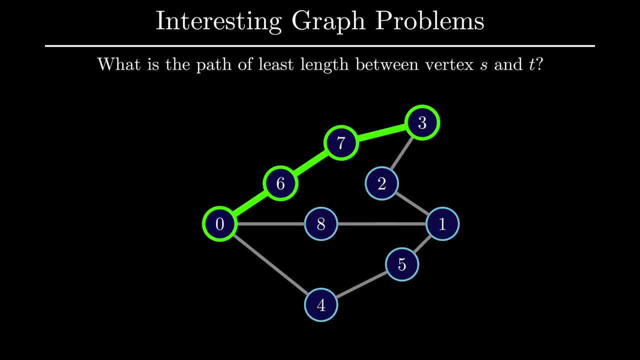 which is something we as humans can generally eyeball for small enough graphs. but, once again, what's the algorithm to solve the problem generally? Then there is a problem of cycle detection in a graph- Many of the algorithms that are used for connectivity problems. 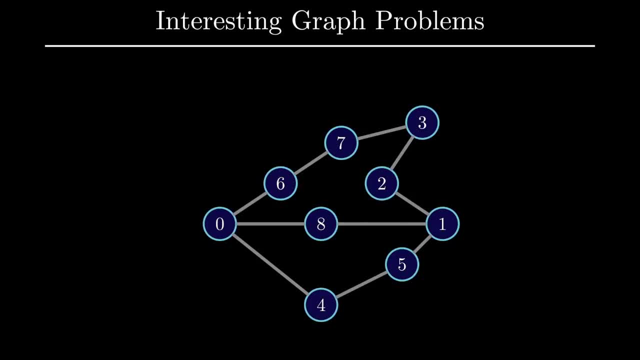 can be naturally adapted to solve this problem as well. Another interesting problem in graph theory has to do with vertex coloring, which we actually saw in the Sudoku example. The problem formally stated is: given a set of colors, can we assign a color to each vertex? 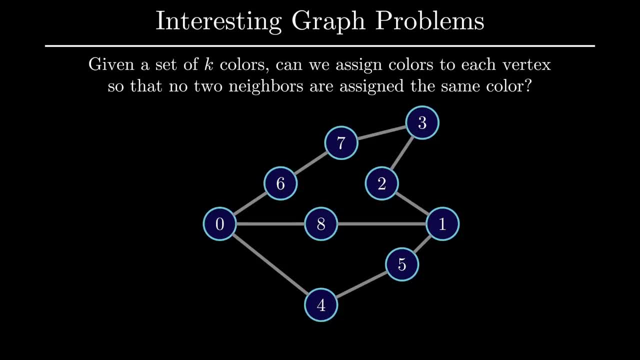 such that no two neighbors are assigned the same color In this graph. for two colors no such solution exists, but if, given three colors, this problem has a solution. Another very interesting problem to ask about graphs is whether a path exists that uses every edge exactly once. 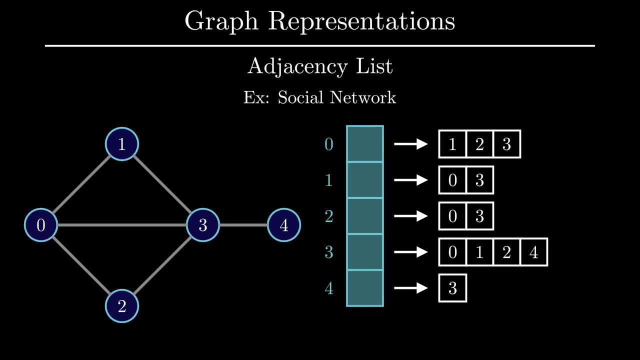 this representation, since there are going to be billions of nodes, but each node is unlikely to have more than a few thousand edges. An adjacency matrix for a graph like that would take way too much memory, but with an adjacency list it's much more manageable. 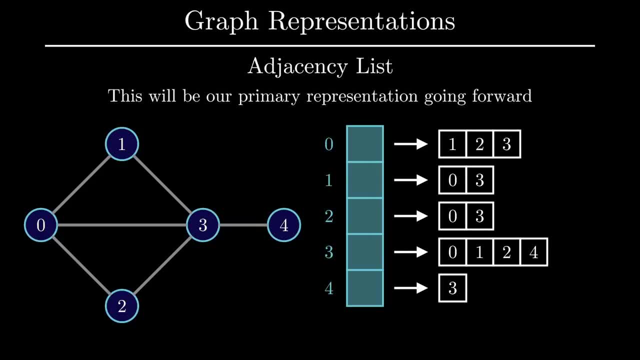 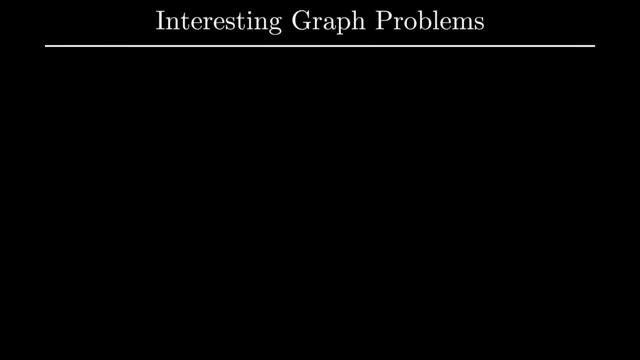 For this reason, in future videos we will primarily use adjacency lists as a way to represent graphs. The final thing I want to do in this video is to discuss some of the interesting problems and questions you may find in graph theory. In future videos we'll show you how you can apply graph algorithms to solve many of these. 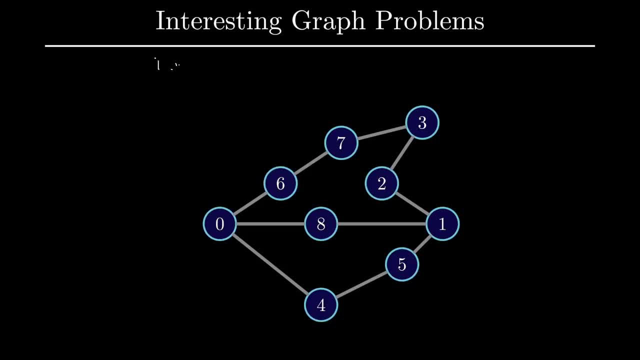 A fairly standard problem that you'll likely encounter all the time revolves around connectivity between two vertices. For example, it's easy for us to see that vertices 0 and 3 have many paths between them, but what sort of algorithms can we use to allow a computer to efficiently solve this problem? 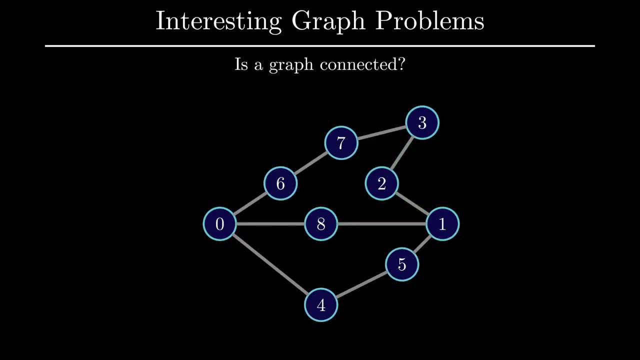 We can naturally extend this problem to ask if an entire graph is then connected. There are a variety of efficient algorithms to solve these problems that we will cover in the next few videos. Another interesting problem in graph theory is the shortest path problem. Specifically, what is the path of the least length between two vertices? 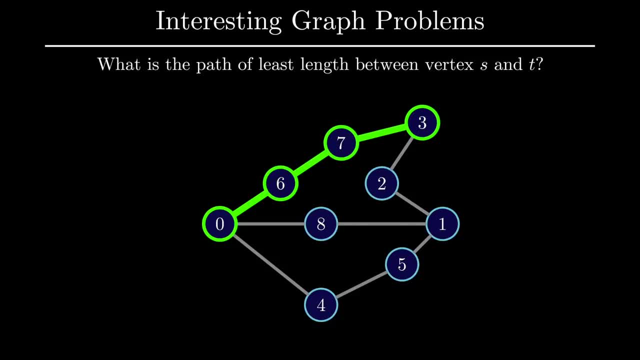 For this particular graph, here is the shortest path between vertices 0 and 3, which is something we as humans can generally eyeball for small enough graphs. but once again, what's the algorithm to solve the problem generally? Then there is the problem of cycle detection in a graph. 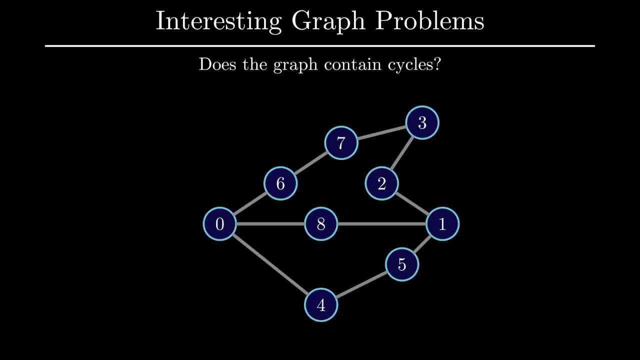 Many of the algorithms that are used for connectivity problems can be naturally adapted to solve this problem as well. Another interesting problem in graph theory has to do with vertex coloring, which we actually saw in the Sudoku example. The problem formally stated is: given a set of colors. 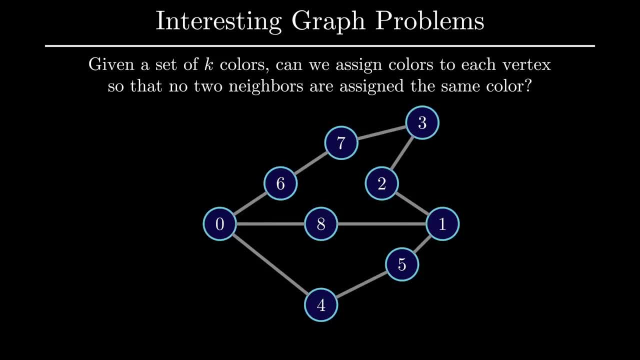 can we assign a color to each vertex such that no two neighbors are assigned the same color In this graph? for two colors no such solution exists, but if, given three colors, this problem has a solution. Another very interesting problem to ask about graphs is whether a path exists. 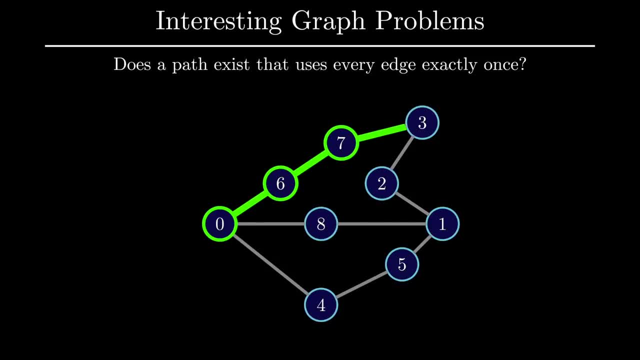 that uses every edge exactly once. It's harder to tell, but this graph does indeed have one of these paths, and an efficient algorithm for this problem exists. These types of paths have tons of interesting applications in bioinformatics and circuit design. A similar question that you may ask is: what about the existence of a path? 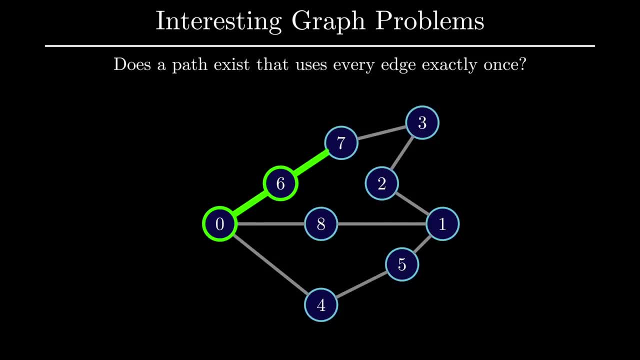 This might be harder to tell, but this graph does indeed have one of these paths, and an efficient algorithm for this problem exists. These type of paths have tons of interesting applications in bioinformatics and circuit design. A similar question that you may ask is whether a path has a path that has two edges. 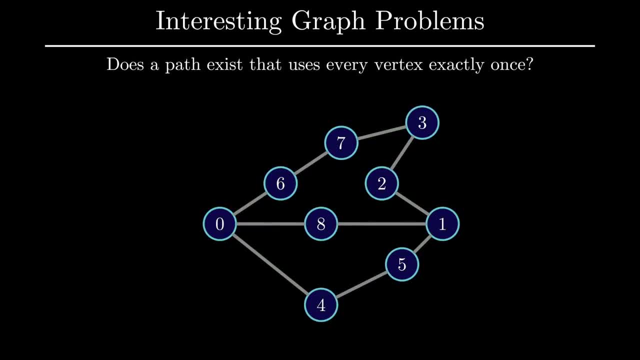 and whether a path has a path that has only one edge. What about the existence of a path that uses every vertex exactly once? Such a path also exists in this graph, but I think what you'll find more surprising is that there exists no efficient algorithms. 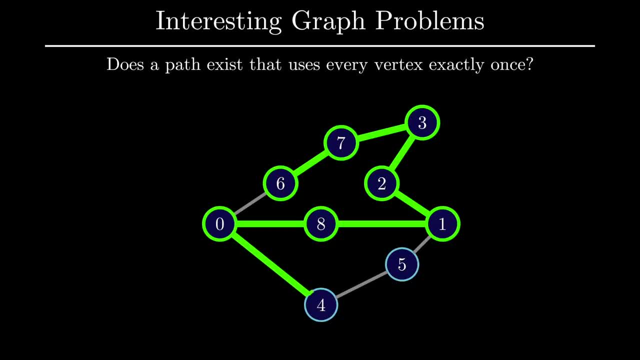 to solve this problem. What I mean by that is that all algorithms that we have so far run in exponential time for this problem, which is incredibly slow for large enough graphs. In fact, if you are able to find an efficient algorithm for this particular problem, 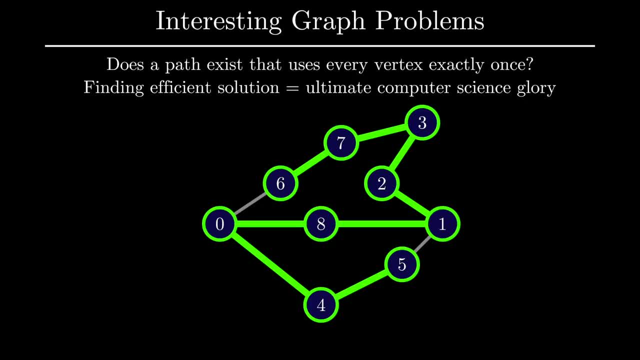 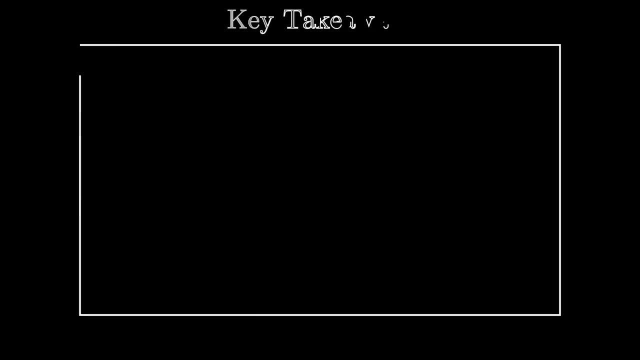 you would probably be given every single computer science award in existence, because it would help resolve a long-standing open problem. But don't get your hopes up there, because there's a fairly large consensus that no efficient algorithm for this problem exists. Let's now take a moment to recap the big ideas in this video. 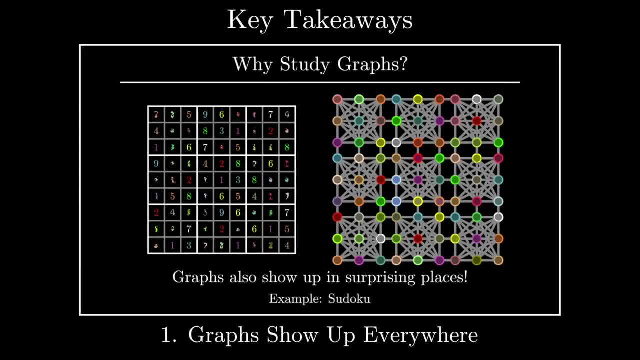 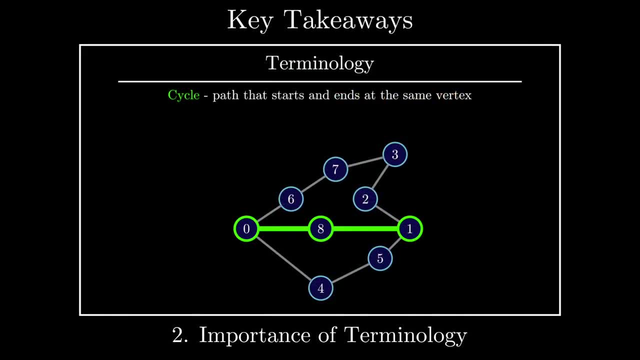 We first introduced graph theory through a variety of cool applications where you saw why someone should even study graph theory. We then formally defined graph theory, along with important terminology and types of graphs that you will encounter. These concepts are incredibly important to understand so that we have an appropriate 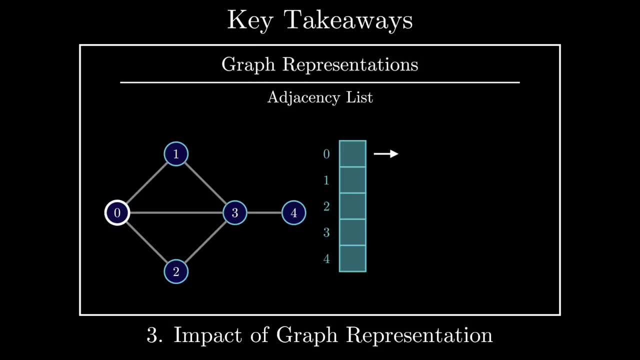 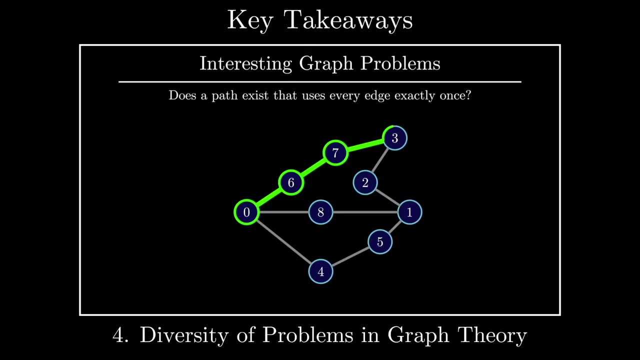 framework for discussing graphs. We then introduced several representations of a graph as a data structure, with the specific emphasis on the practicality of the adjacency list, And, lastly, we introduced some diverse and interesting problems in graph theory to motivate the algorithms that we will go through in future videos. 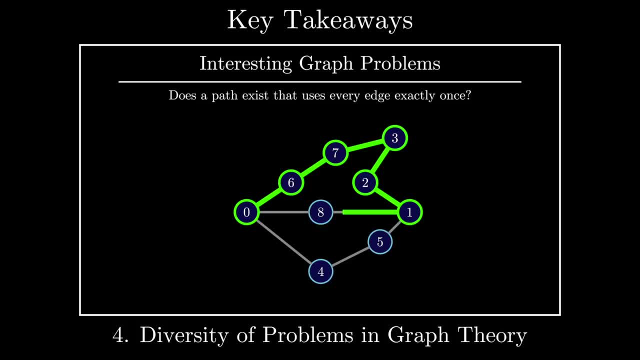 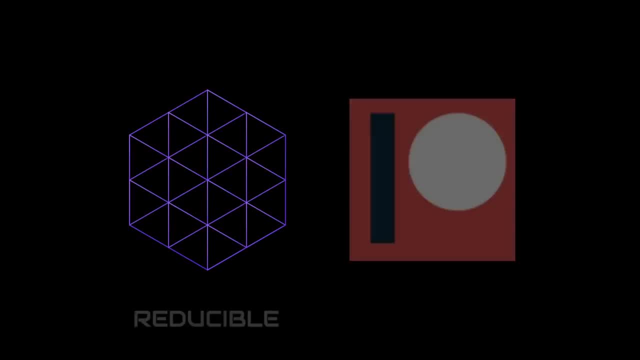 I hope this discussion gave you an appreciation for the massive field of graph theory. It's definitely one of my favorite topics in computer science and I hope it becomes yours as well. Thanks for watching me and, as always, I'd appreciate it if you hit the like button if you enjoyed it. 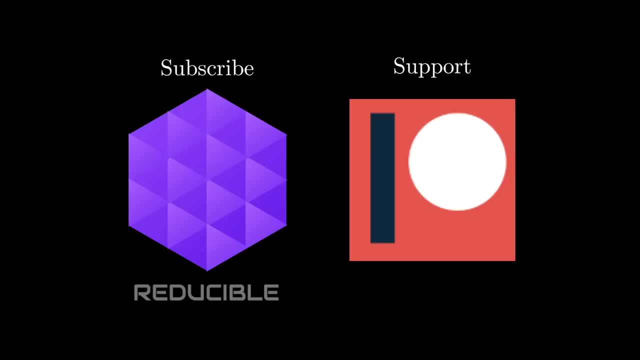 If you want to see more content like this, be sure to hit the subscribe button, And if you want to more directly support this channel, be sure to check out the Patreon page linked in the description below. See you in the next video. 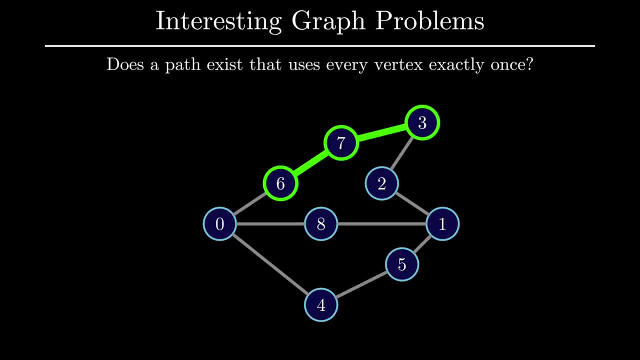 that uses every vertex exactly once. Such a path also exists in this graph, but I think what you'll find more surprising is that there exists no efficient algorithms to solve this problem. What I mean by that is that all algorithms that we have so far run in exponential time. 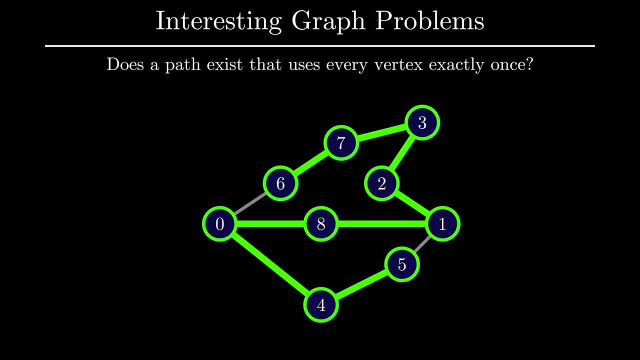 for this problem, which is incredibly slow for large enough graphs. In fact, if you are able to find an efficient algorithm for this particular problem, you would probably be given every single computer science award in existence, because it would help resolve a long-standing open problem. 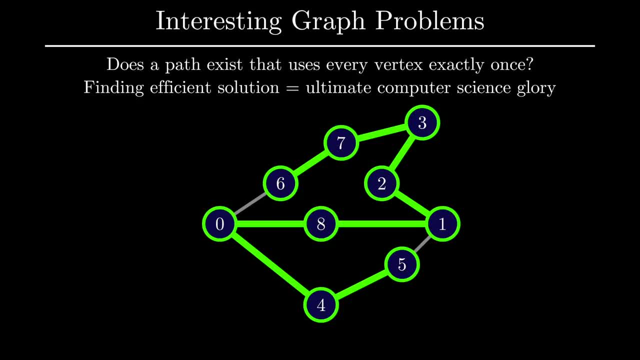